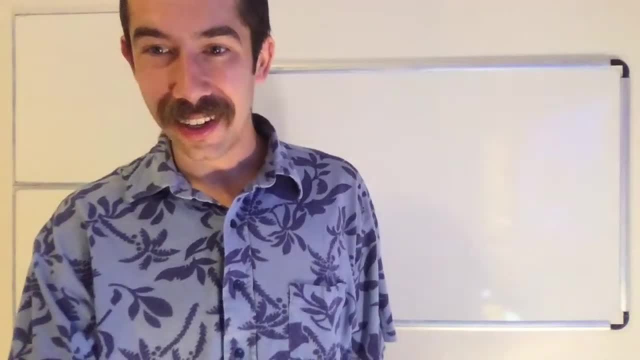 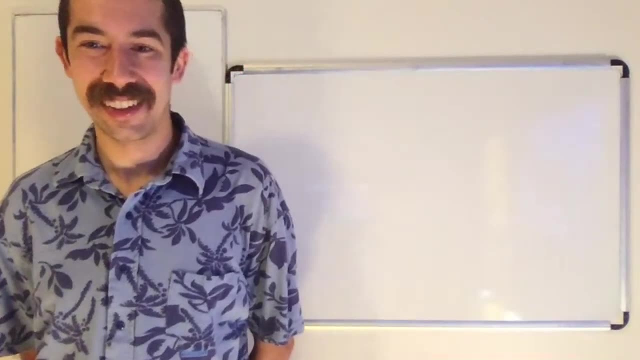 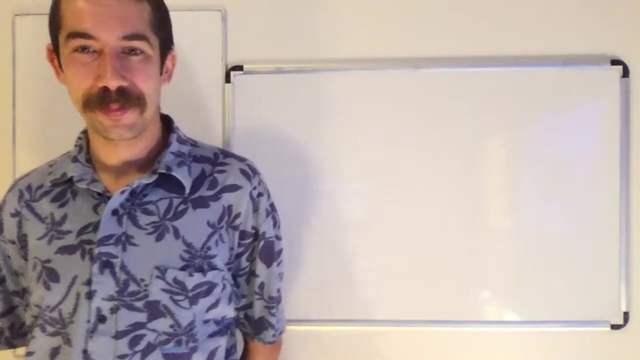 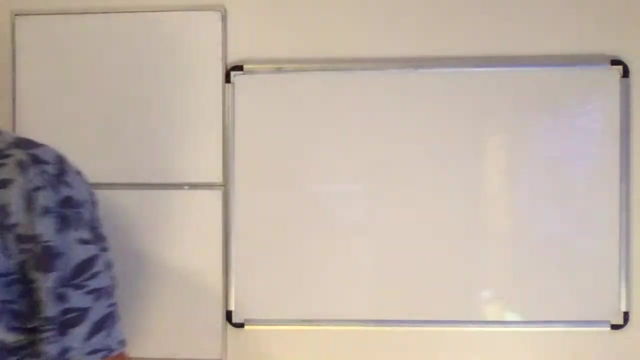 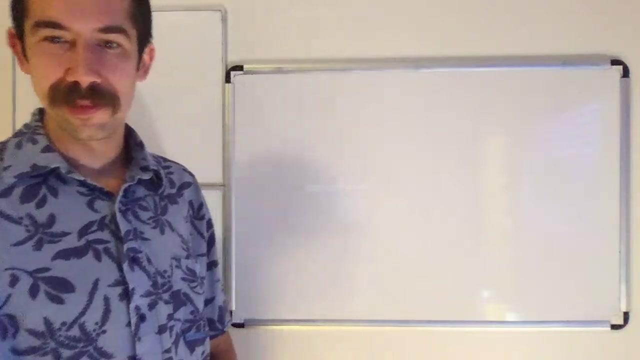 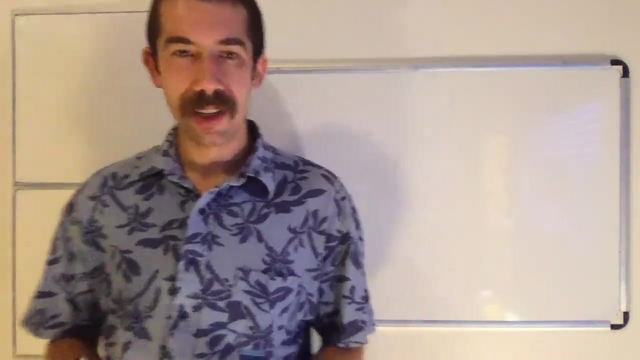 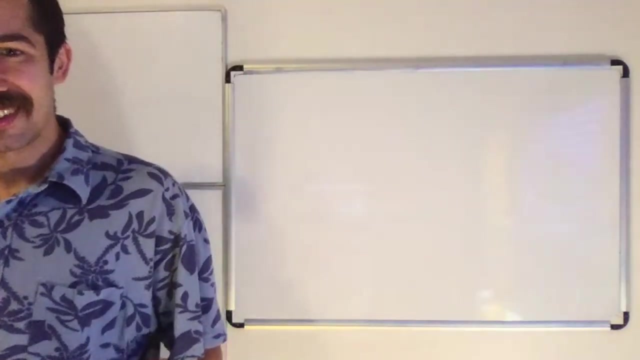 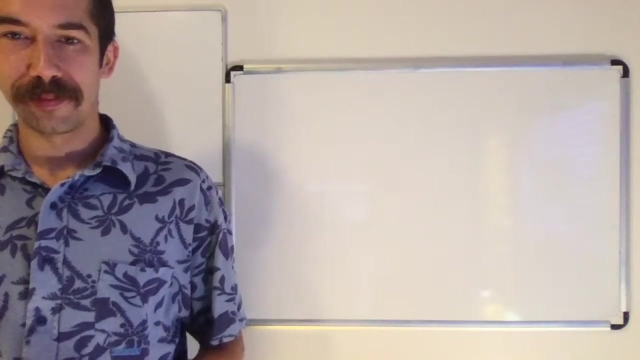 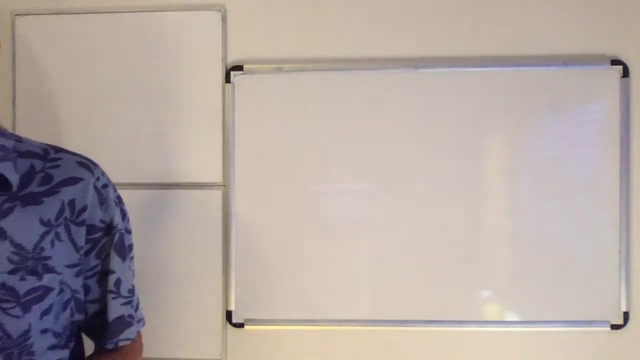 Hello, Hello. I'm not sure who said evening from China, but hello. Good morning Emma. We'll get started in I don't know a minute or so. Hopefully a few more of you trickle in. Good morning Shu Tong, Glad you're here. 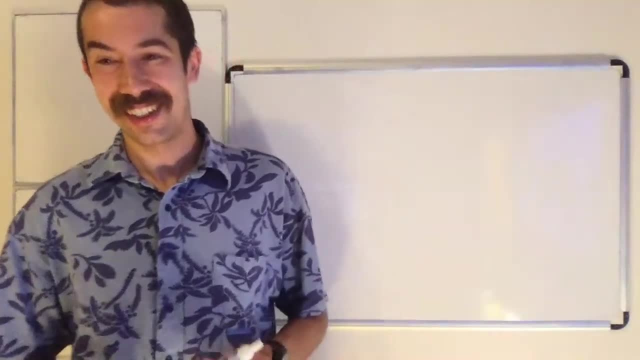 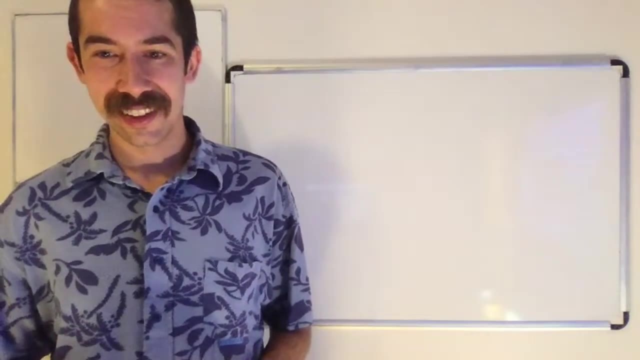 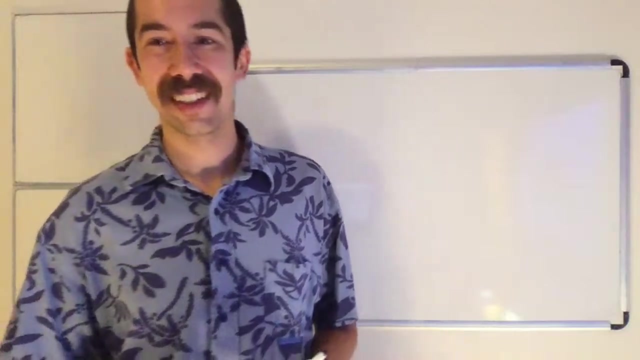 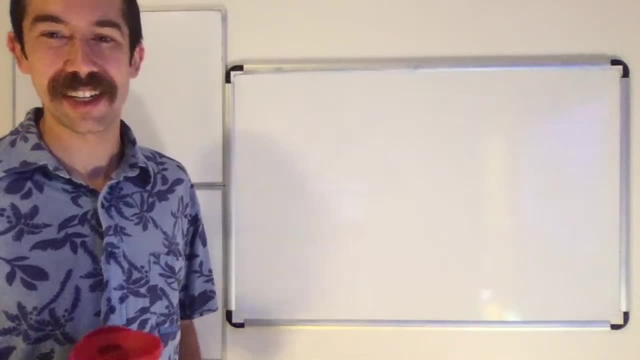 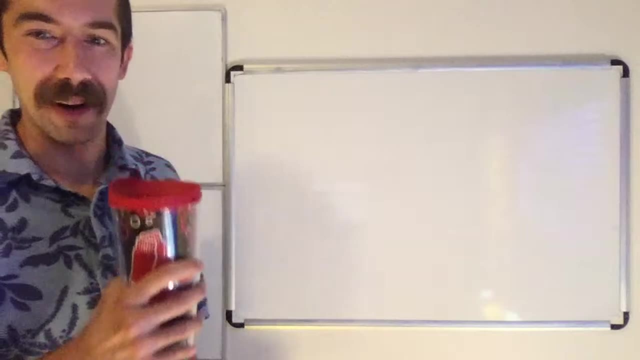 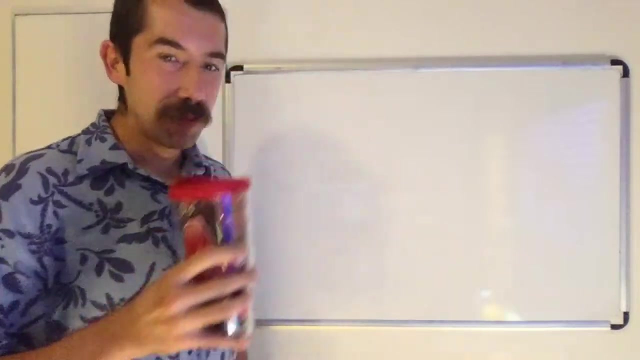 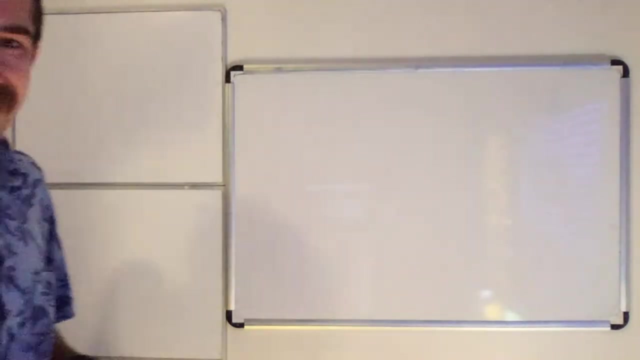 Oh, it looks like Sue was in the chat just in time for the simultaneous sip. So if you have your coffee or your water or your tea or whatever you may have, feel free to join me in the simultaneous sip. All right, let me see in the chat who joined in on the sip this morning. 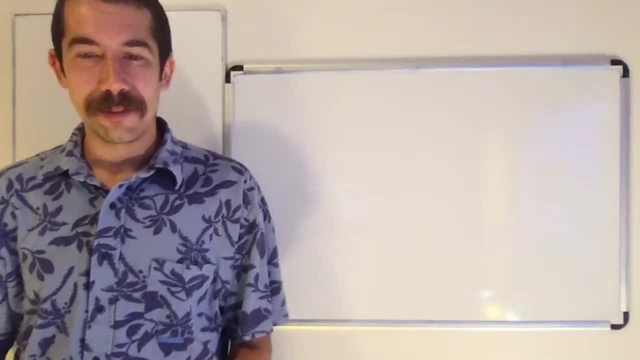 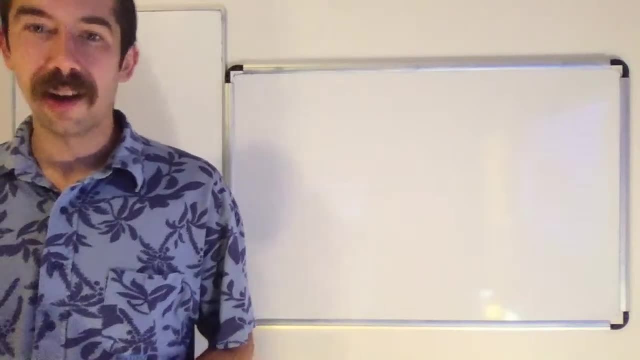 But the plan for today and basically the rest of this week, is we're going to keep working on this, All right. So we're going to be talking about inner product space section, All right. So I know yesterday's class was a little bit theoretical. 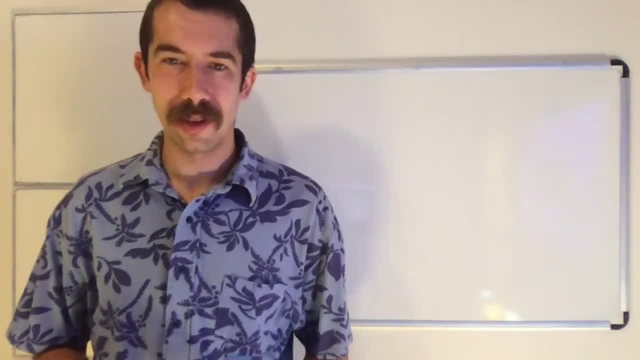 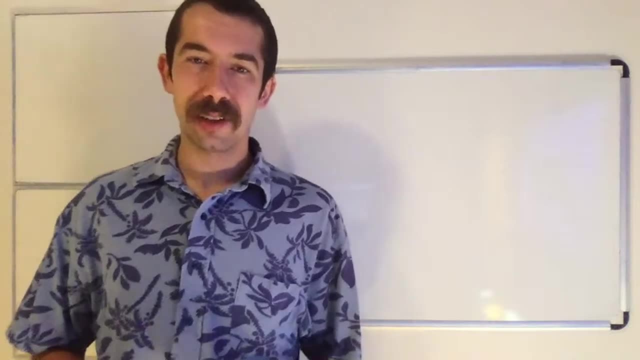 So today we'll see some more examples of how we're going to use these concepts, But slow me down if I'm going too fast. We have not a ton of material left for this semester, but we still have what five classes. 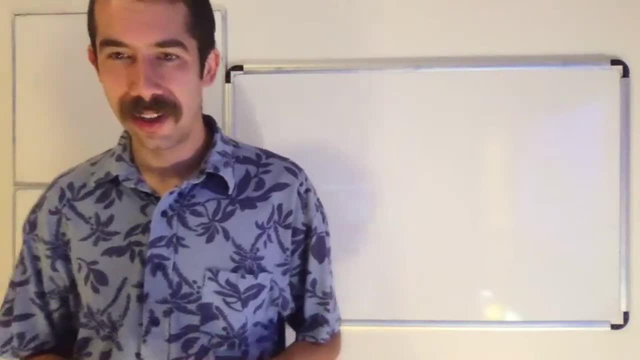 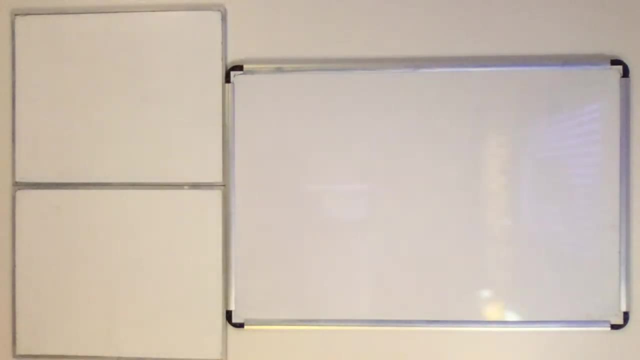 So slow me down if we're going too fast. All right, nice, We've got a few people joined in with the sip today. Excellent, Excellent, All right, Okay. so we said at the end of class yesterday we could use these inner products to define the length. 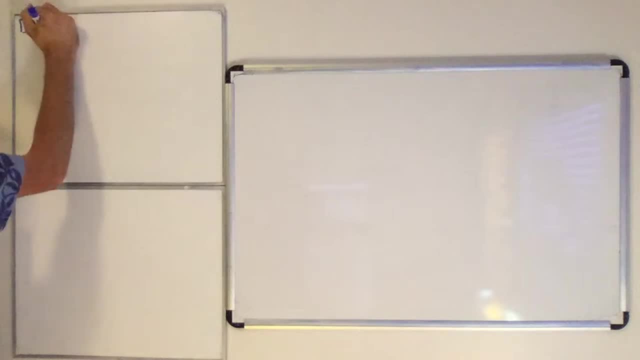 So just some more definition. A unit vector is one whose length is one. So it's a vector not in the column vector sense but in more of the theoretical vector space sense. So we'll see. If a polynomial's length is one, we call it a unit vector. 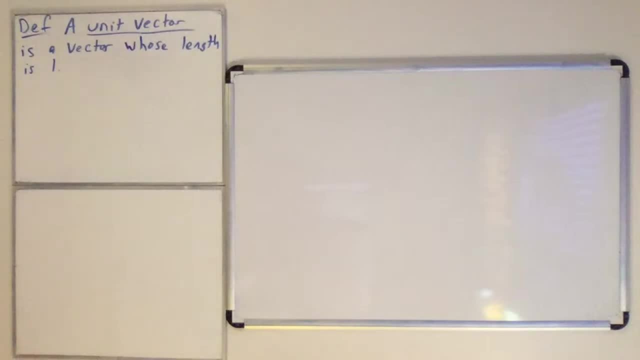 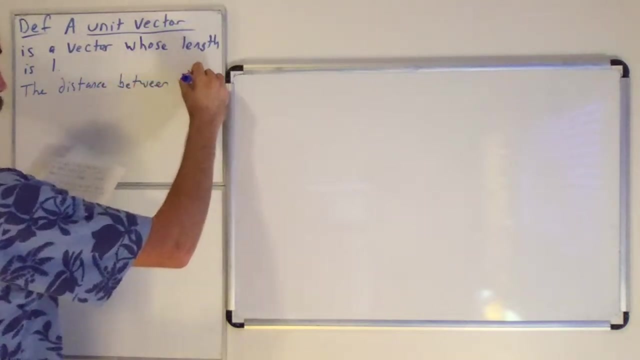 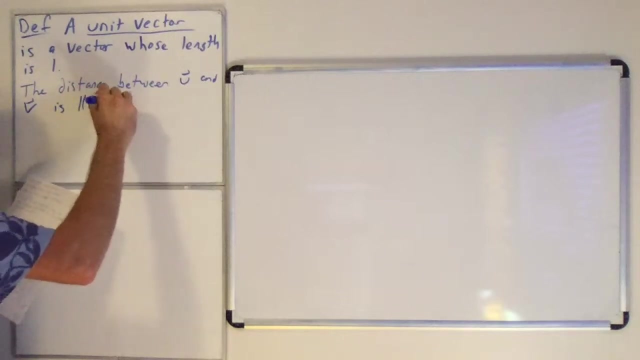 All right. so if we take the inner product with itself and we get one, then we have a unit vector And, just like before, the distance between two vectors is the length of u minus v. But here again we're going to be using length in terms of our inner products. 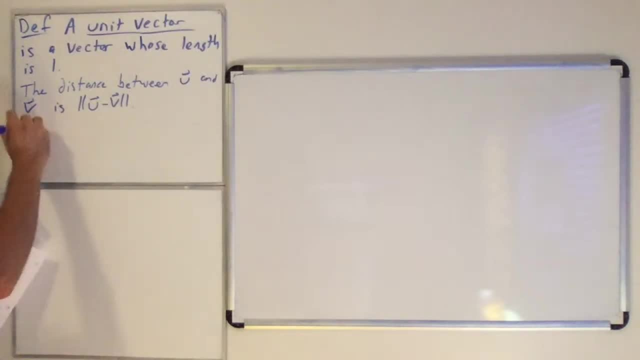 And then just one last bit: Vectors u and v are orthogonal. Okay, how do we think we test to see if two vectors are orthogonal? Let me know in the chat. Bye, Bye, Bye, Bye, Bye. So two vectors, u and v, are orthogonal if – yeah, see, Chai, you'd want to say the dot product. 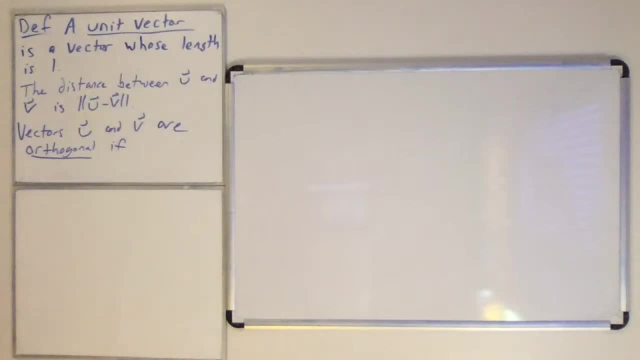 but we're talking about the inner product now. But yeah, Taylor, you're right. So if their inner product is zero, Right, because we don't really know what it means. to take the dot product of two polynomials, for instance: 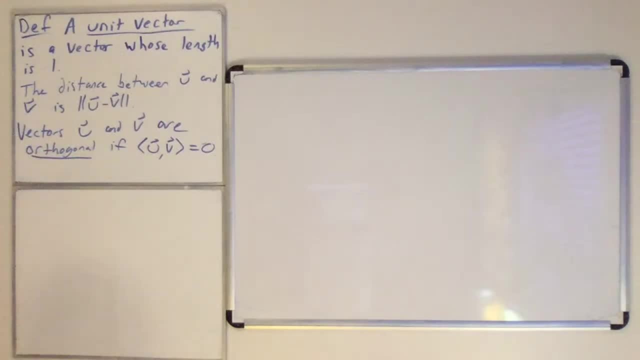 But you know we could – we'll use this term orthogonal just to mean that their dot product – or their inner product is zero. Okay, let's look at an example. So we'll let P2 have the inner product. Let's look at that. 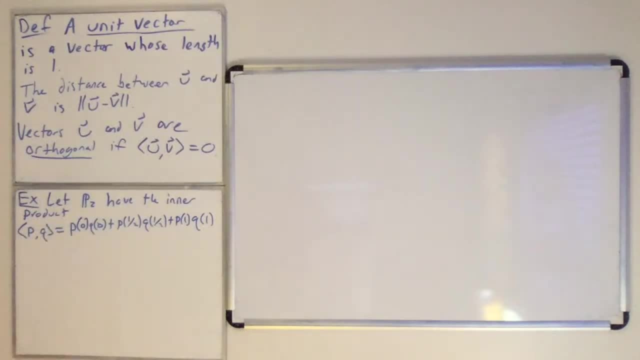 Q have the following inner product: So this is the one we looked at yesterday: P of zero times Q of zero plus P of one-half times Q of one-half plus P of one times Q of one. Okay, The question is compute – compute the lengths of – 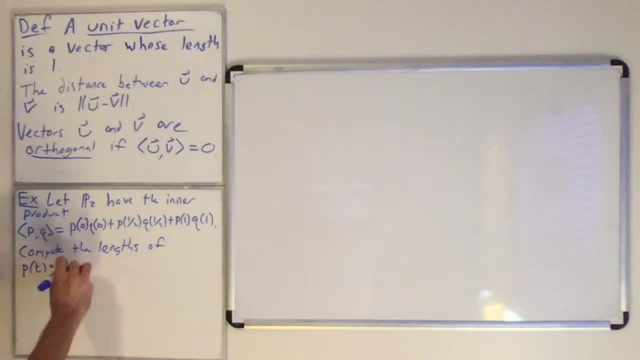 P of T, which is equal to 12 T squared Q of T, which I think we already did yesterday but do it again, which is 2T minus 1.. And P minus Q of T. So this is really going to ask us how close are these two polynomials in this inner –. 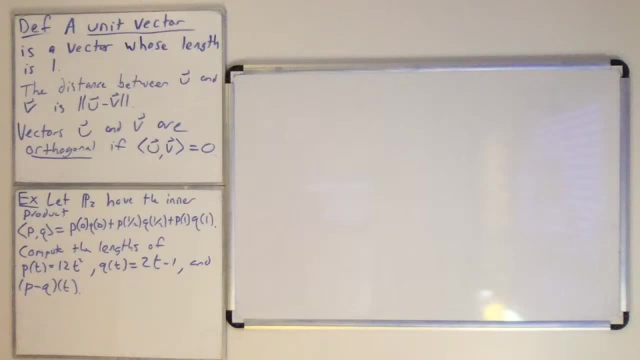 in the sense of this problem, In the sense of this inner product. Okay, so I'll give you, let's say, a minute and a half or so to try to work this out. Does somebody in the chat want to say how they're going to compute these lengths? 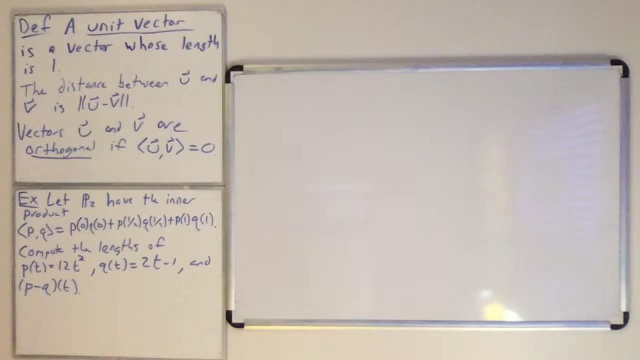 Yes, Okay, so I'll give you a minute or so to try to work this out, Okay, And if you get an answer, feel free to share it with the chat. Okay, All right. Taylor said something For p minus q. do we have to do p minus q dotted with itself? 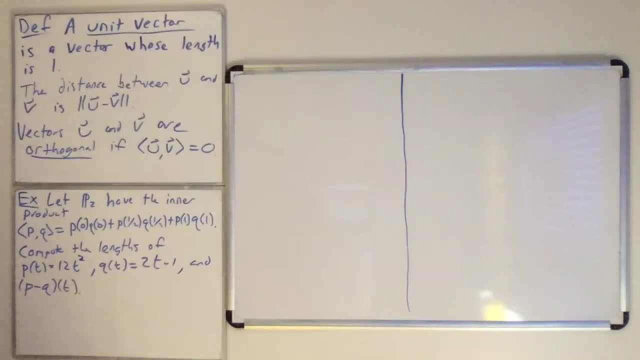 Yeah, So we would have to figure out what is the polynomial p minus q. So that would just be 12t squared minus 2t plus 1, right, because we subtract this whole thing And then, yeah, take the inner product with itself. 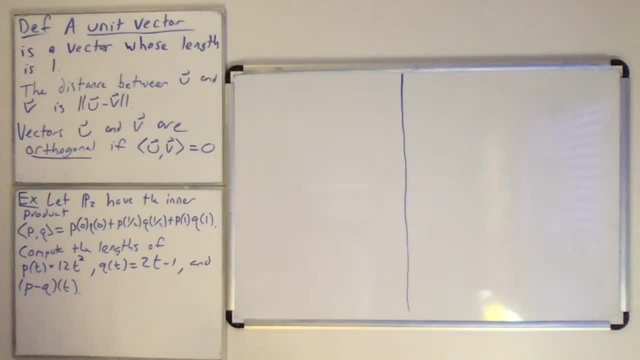 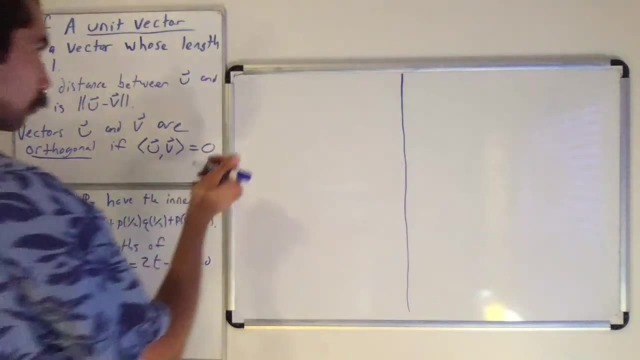 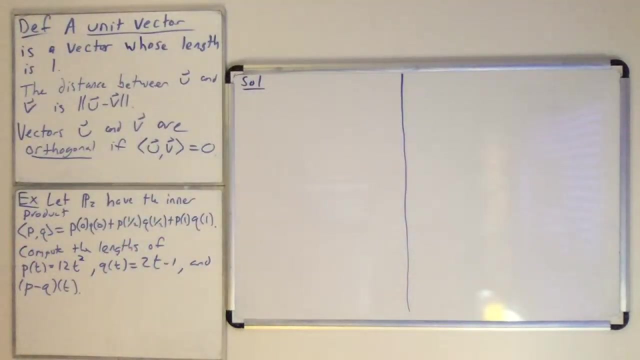 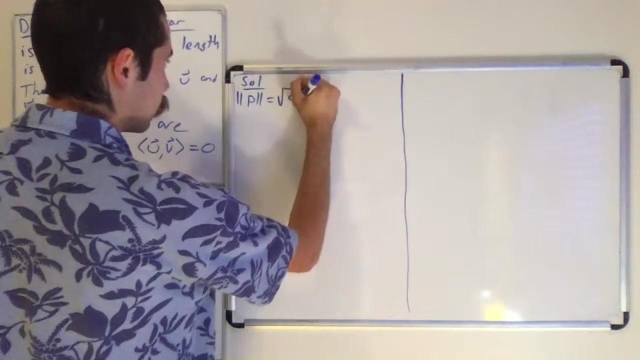 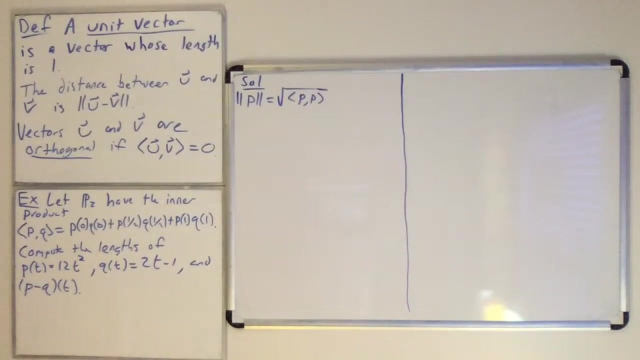 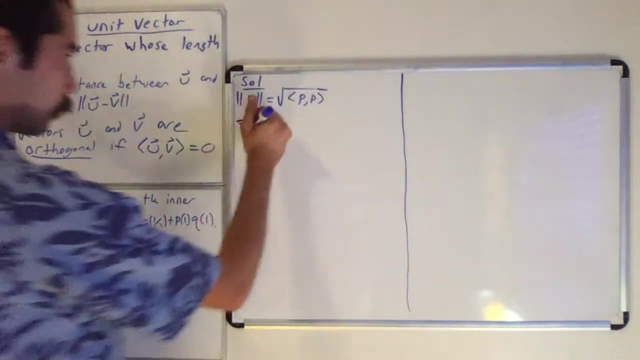 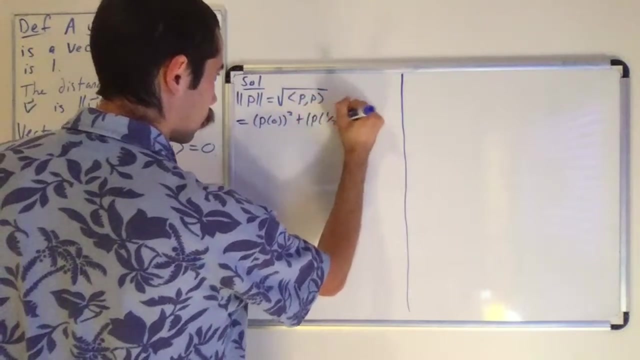 and, And then take the square root of that inner product. Okay, So to find the length of these vectors, the length of p is equal to the square root of p with itself, Which is equal to p of 0 squared plus p of 1 half squared plus p of 1 squared. 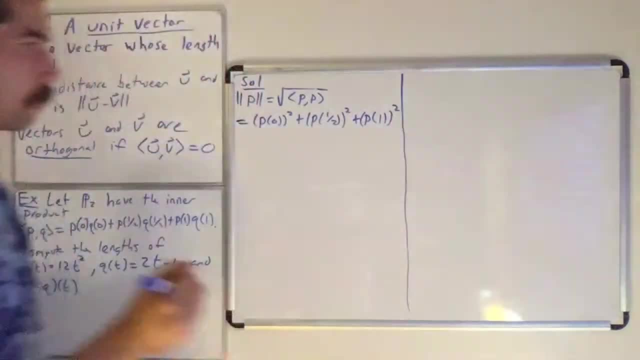 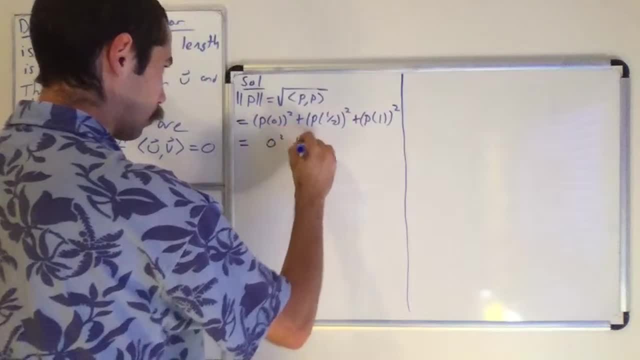 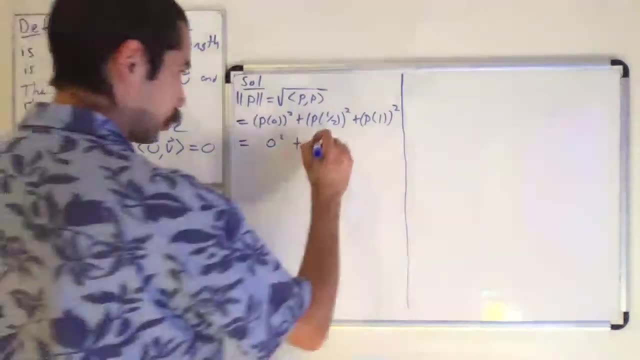 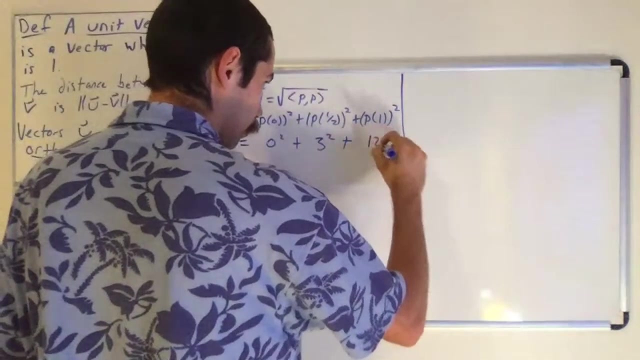 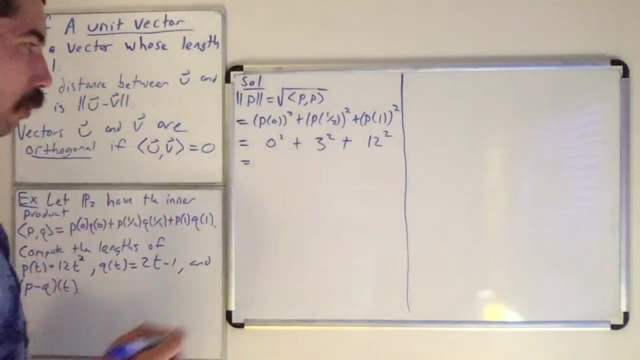 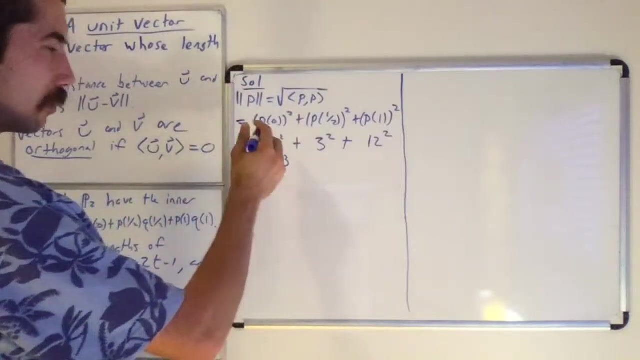 Oh, Oh, Oh Oh, P of 1 half is 3. And p of 1 is 12.. So 0 plus 9 plus 144 is 153.. And, And I guess we should be taking the square root of all this, 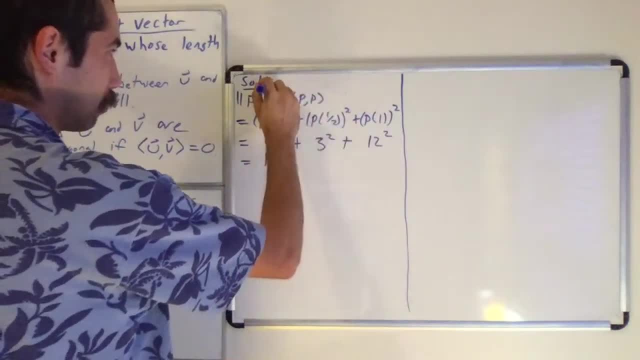 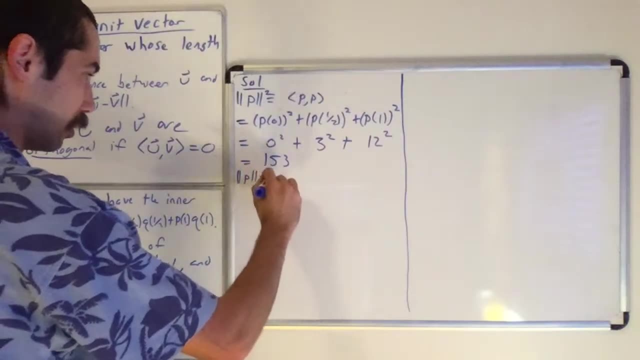 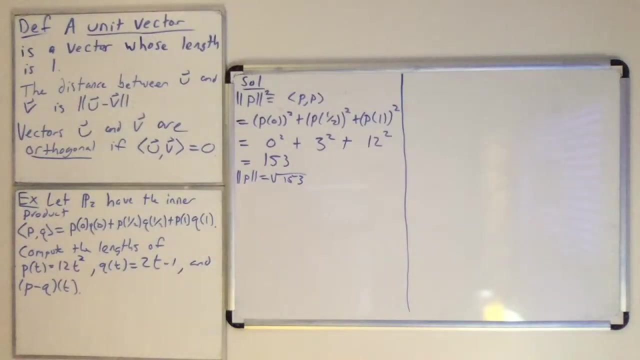 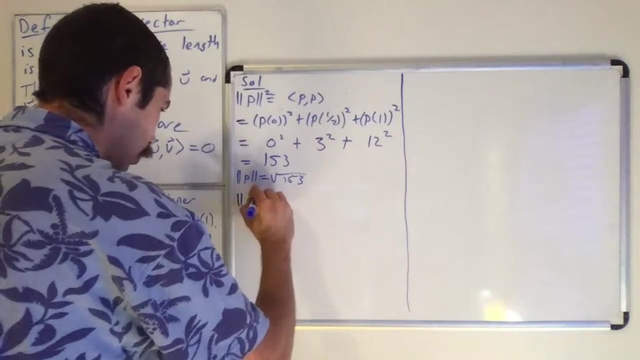 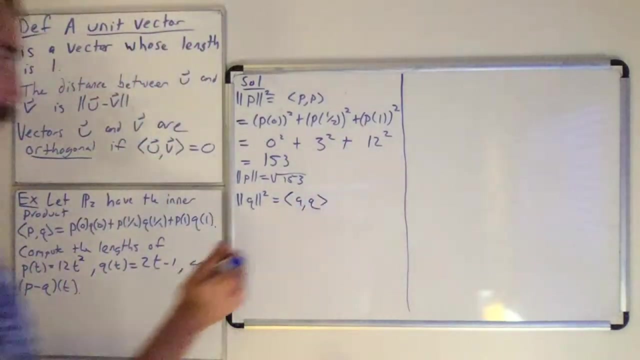 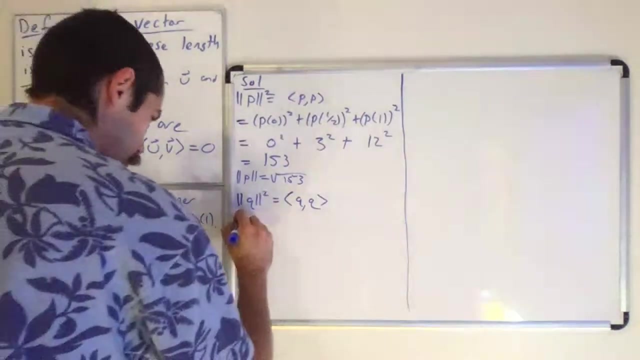 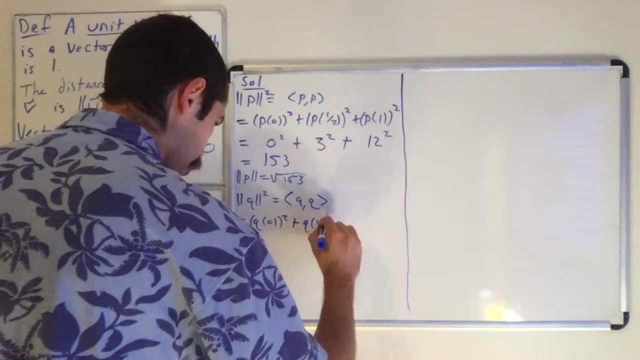 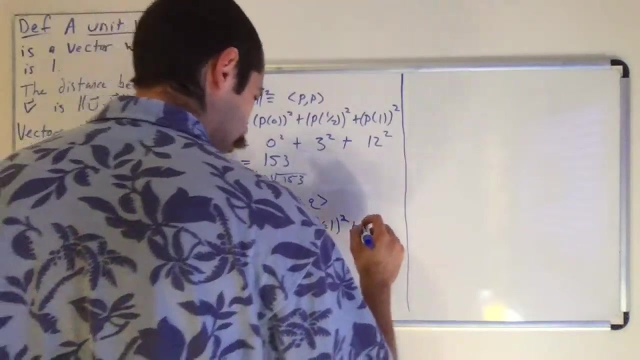 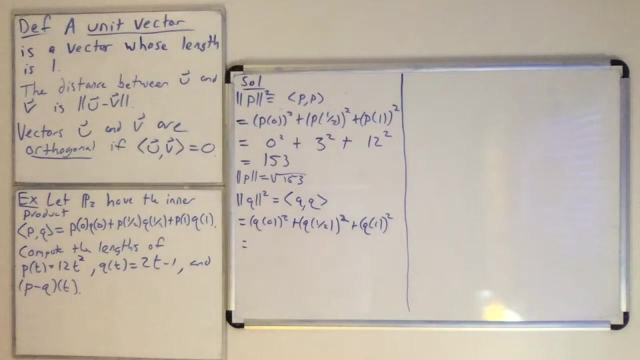 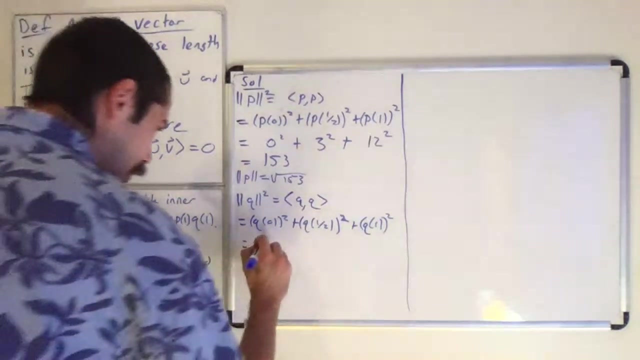 So let's correct this. And so if the magnitude squared is 153, the magnitude of P is the square root of 153.. All right, similarly for the magnitude of Q squared, which is Q inner product with itself. All right, When we do this, we get negative 1 squared plus 0 squared. 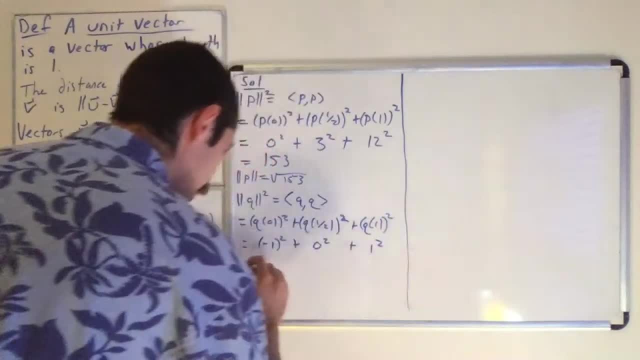 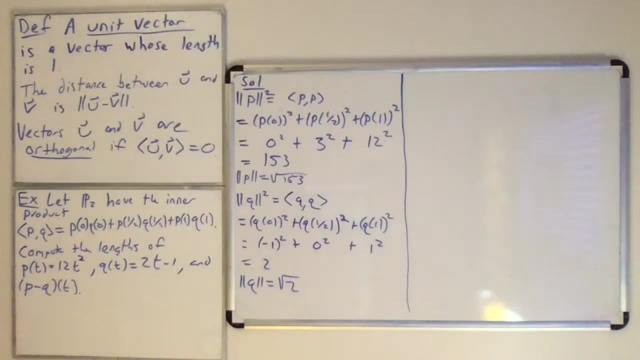 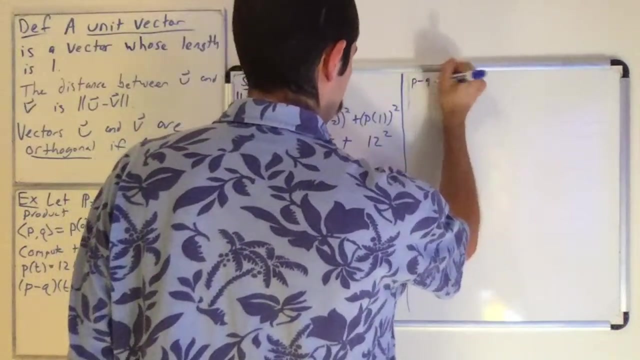 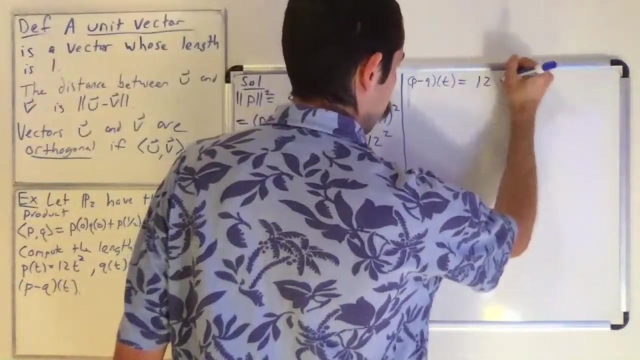 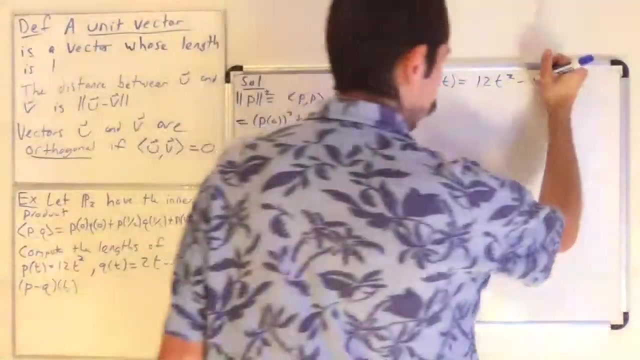 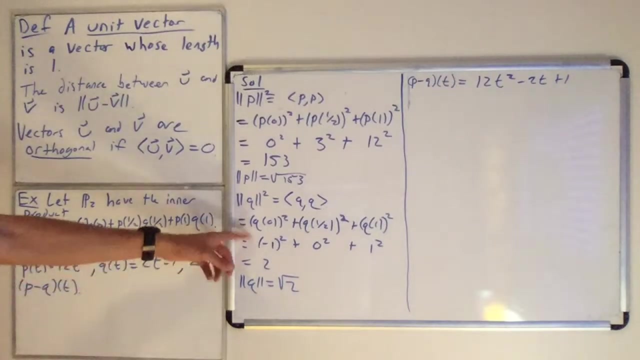 Plus 1 squared, which is 2.. So the magnitude of Q is the square root of 2.. And then last, P minus Q is the polynomial 12T squared Minus 2T plus 1.. I guess to evaluate its inner product we need to evaluate it at 0,, 1, half and 1.. 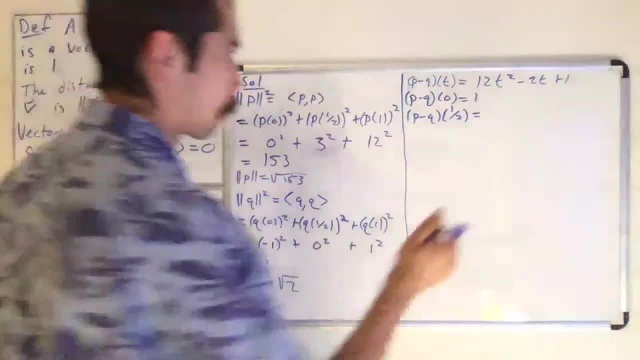 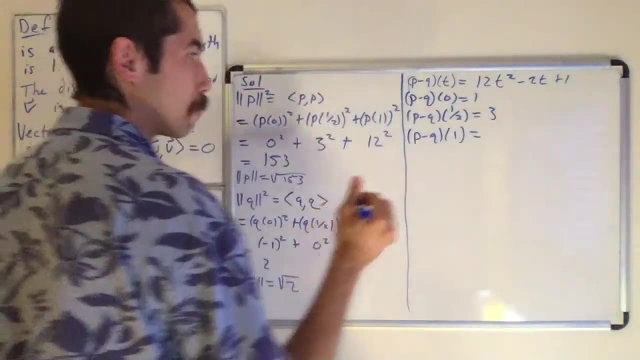 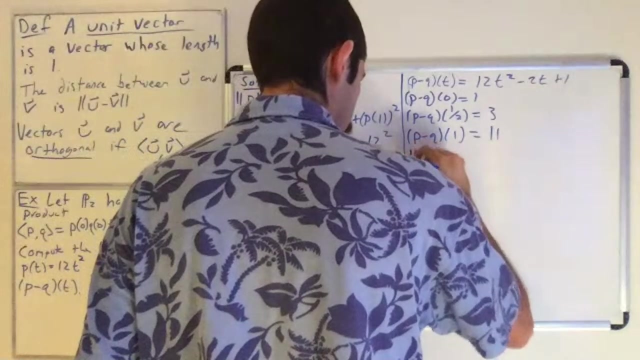 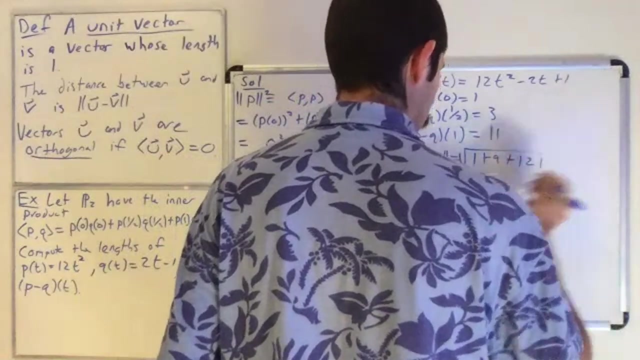 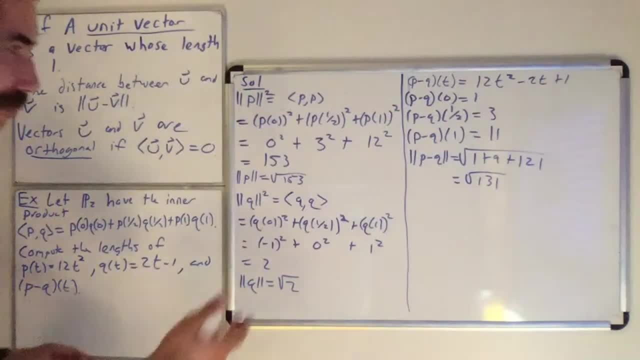 All right, All right. So in the sense of this inner product, the distance between the polynomials P and Q is the square root of 131.. So can I get a little feedback from you all in the chat Whether this idea of finding the length of a polynomial given an inner product is one that 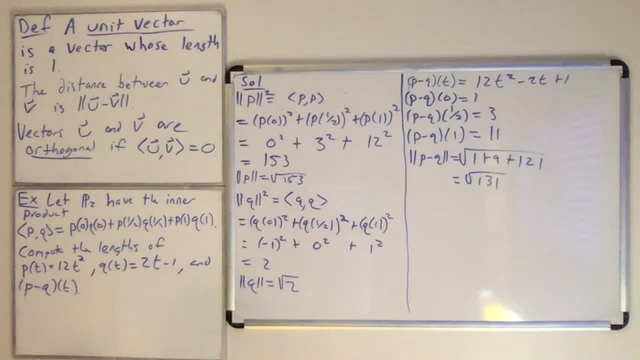 you understand, or maybe you need a little bit more clarity for All right, A couple of thumbs ups. All right, That's good. That's good, All right. And given a different inner product, maybe these polynomials would have a different length. 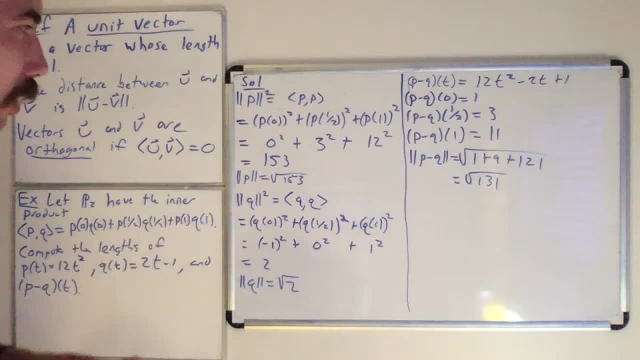 We'll see some applications where you're given. you know, let's say, you're in the lab and you want to find the line of best fit or the curve of best fit and you're given some data points. That would be this information here. 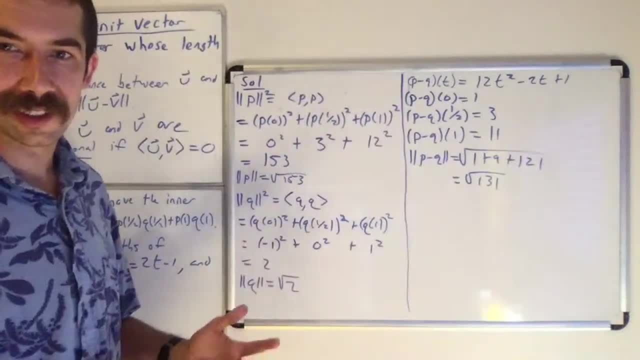 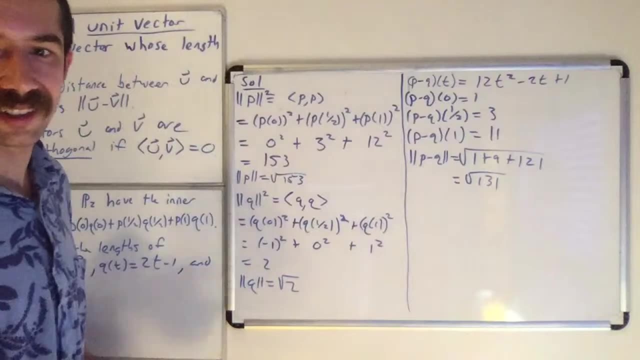 And you want to ask: you know which polynomial matches this data the best? You'd want to minimize some sort of distance here. We're going to talk about how to do that in a second. But this stuff has applications in, you know, the field of data science or statistics. 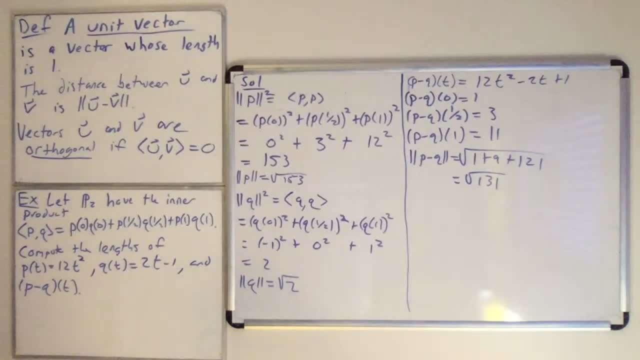 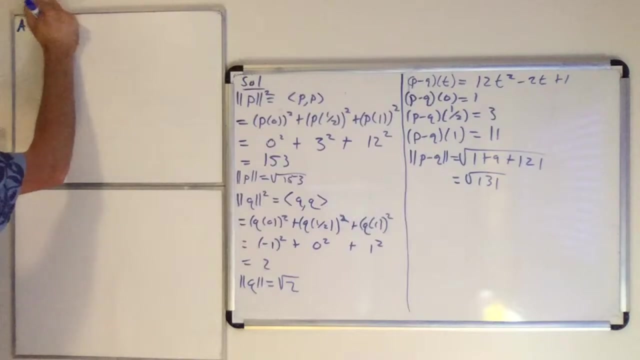 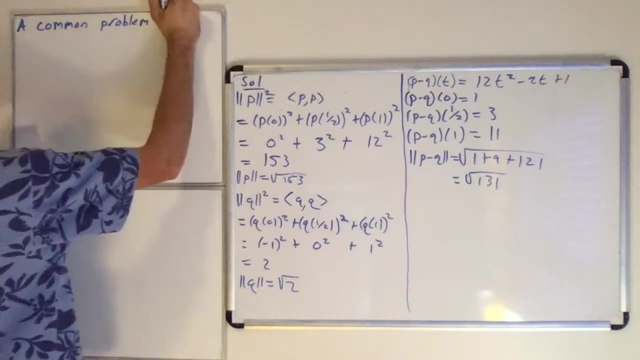 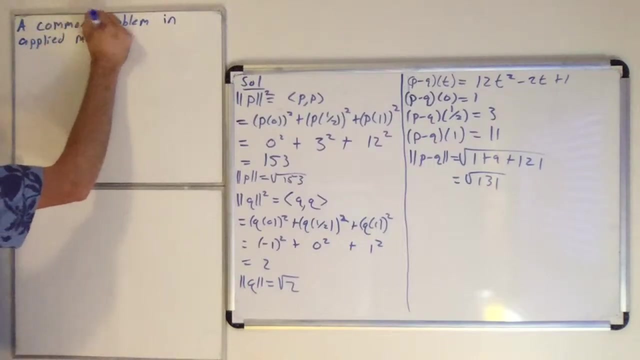 That's pretty useful. So we'll take a look at that, hopefully in a few days. Okay, So let's talk about that a little. So a common problem in applied math Involves a vector, space V, whose elements are functions, maybe not polynomials, but continuous functions or just functions. 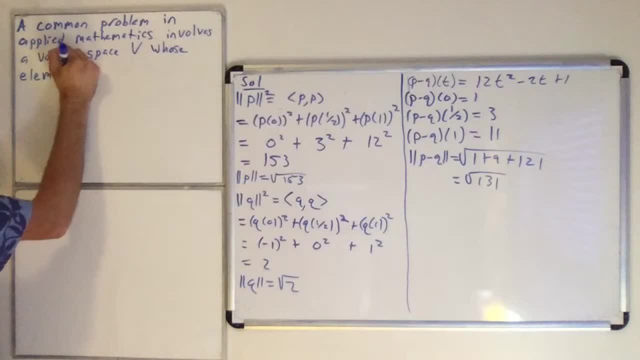 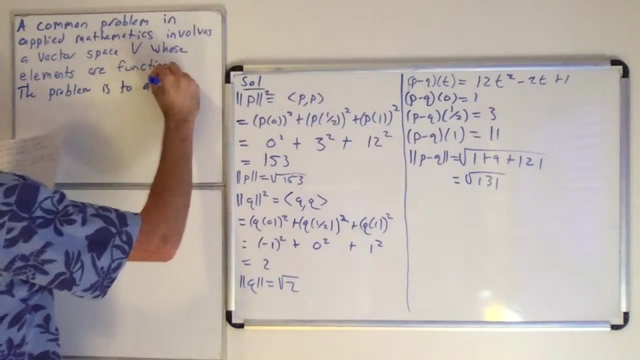 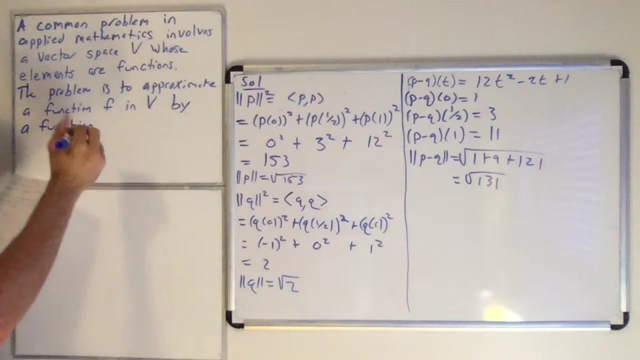 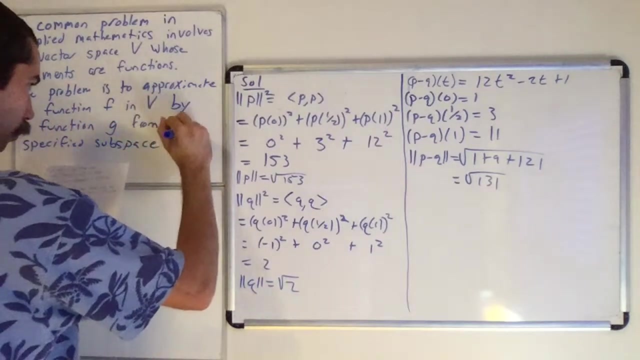 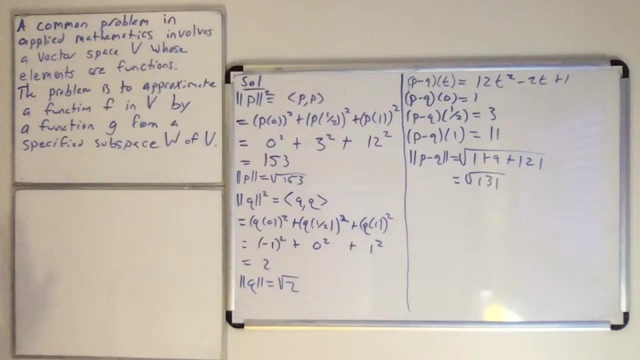 The typical problem you'll try to solve. So the problem is to approximate, Okay, A function f in V By a function g in some subspace, Okay, And we have a subspace that we particularly like. Okay, So before we write anymore, 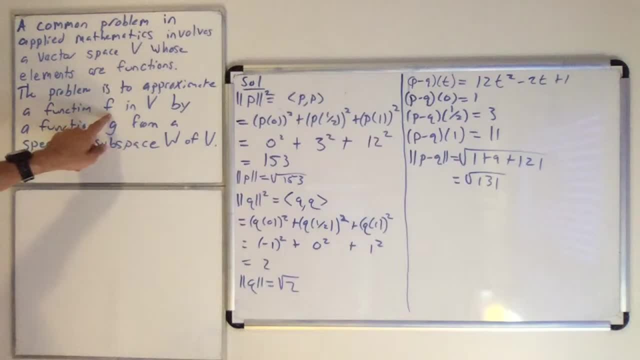 Basically, we're given some function, f, And we have a subspace that we particularly like, Like, for instance, This: This polynomials, And we want to ask which polynomial is most like F? Okay, You've actually seen this before if you've taken Calc 2.. At least at NC State we taught this, So let me see. 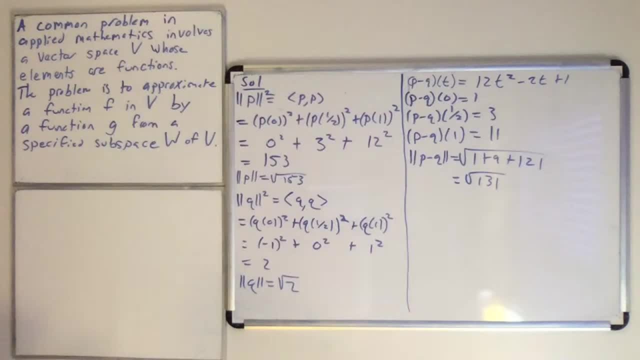 in the chat. have you done like Taylor expansion or Maclaurin series, Taylor or Maclaurin series when you took Calc 2? Is that familiar? At least you've heard of it before. Yeah, it was the last chapter, Yeah, so that's kind of the idea of what you're doing. You have 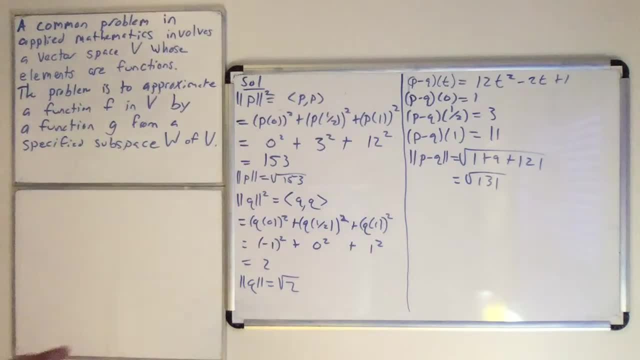 a function and you're approximating it with a polynomial, And in calculus you had some kind of procedure to find that polynomial. But maybe we're going to deal with an inner product. that's a little different, So our procedure will be slightly different. We're 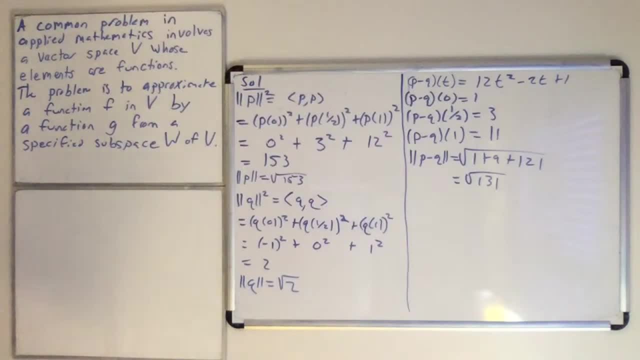 going to deal with an inner product. that's a little different, But if we restrict it the appropriate way, we could get back that Taylor series. Okay, So that's kind of the idea. Okay, so we're going to consider a case where the length of the distance, so how far? 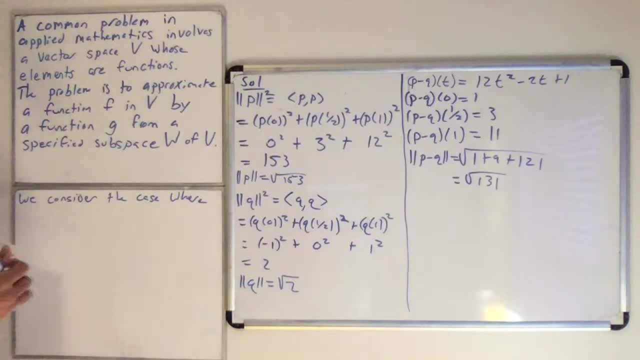 away F and G are is determined by an inner product. Okay, so we're going to consider a case where the length of the distance, so how far away F and G are, is determined by an inner product. Okay, so we're going to consider a case where 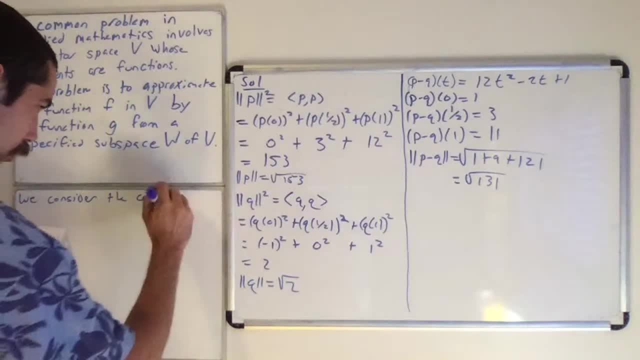 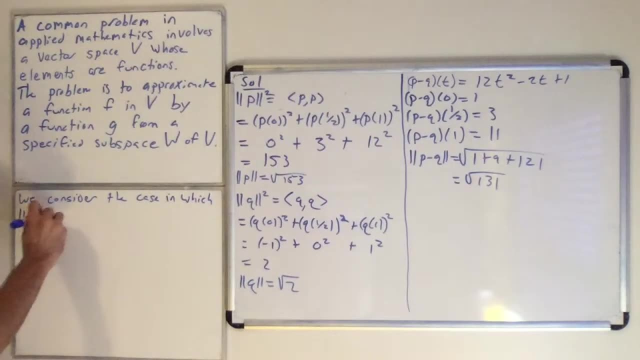 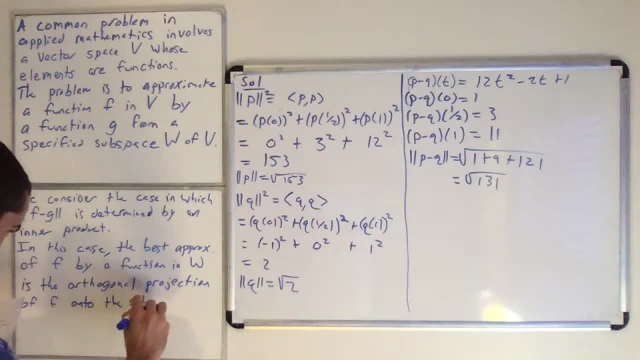 the length of the distance. so how far away F and G are is determined by an inner product. All right, so what we did in our last section orthogonal projections – it's going to appear again, but now look at this not in the sense of column vectors, but in a sense. 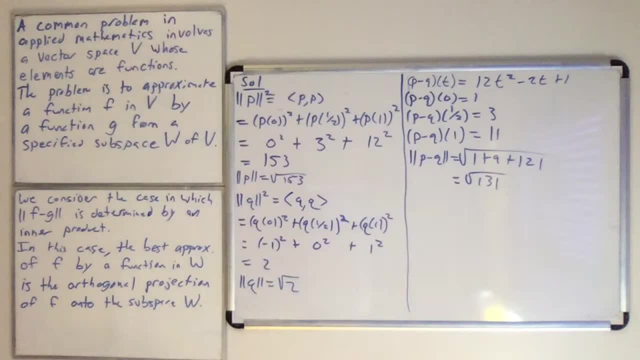 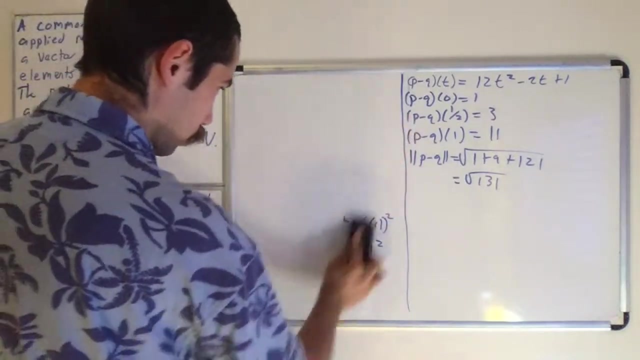 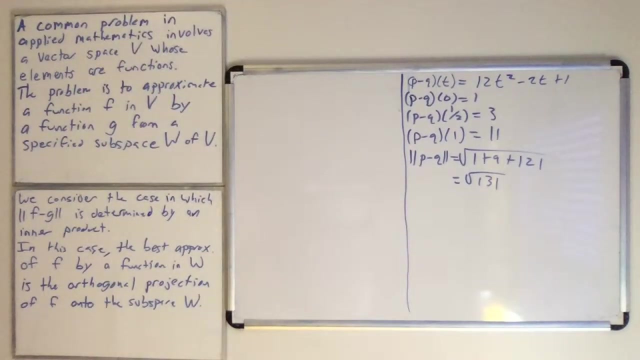 of a general vector space. Okay, so what did we do? OK, so let's take a look at an example to see that what we're doing here is really not too bad. OK, so this example has two parts, So we'll just do one part at a time. 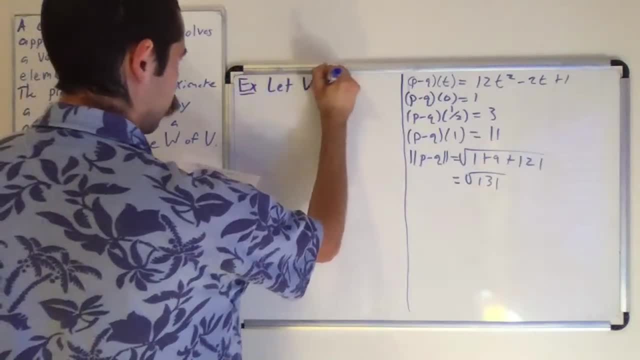 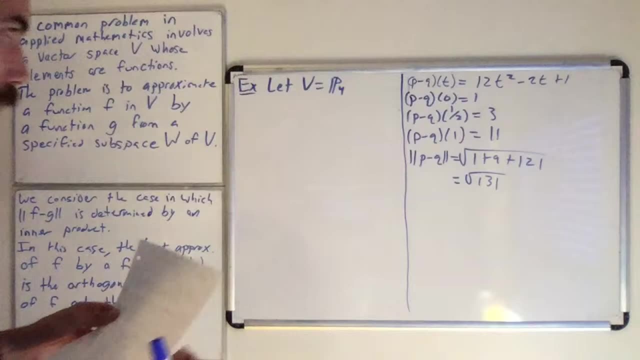 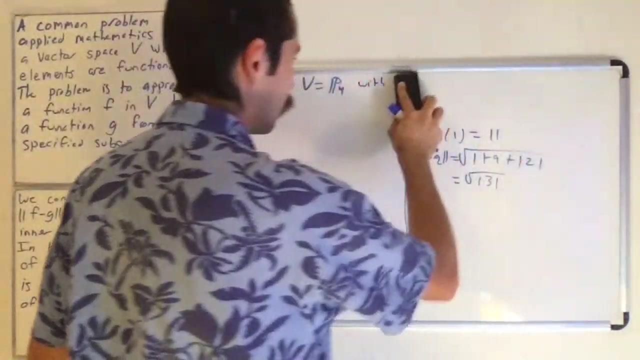 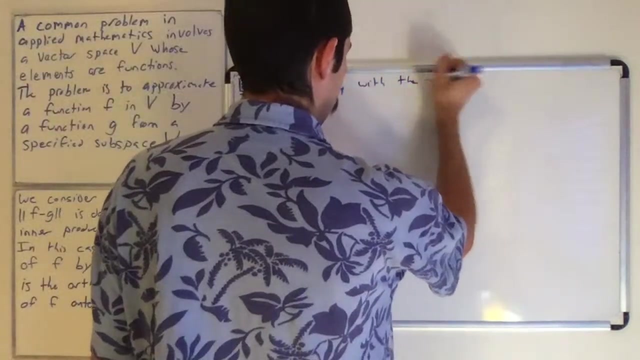 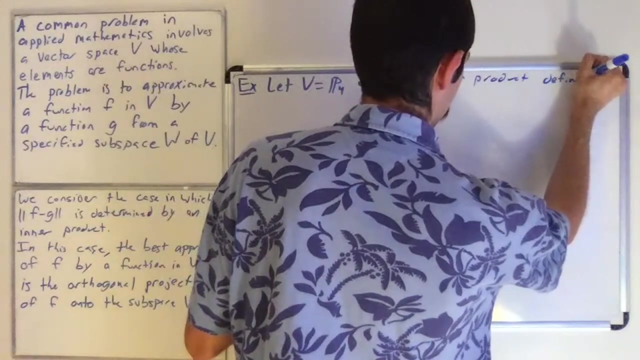 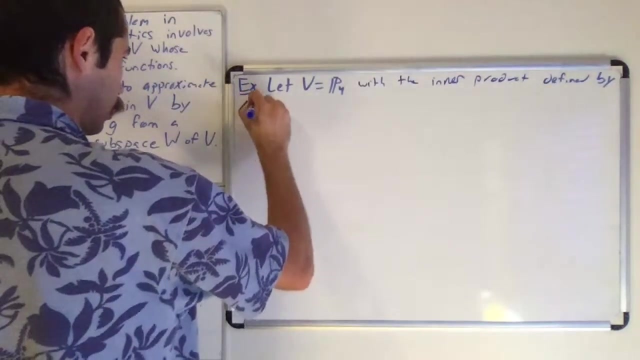 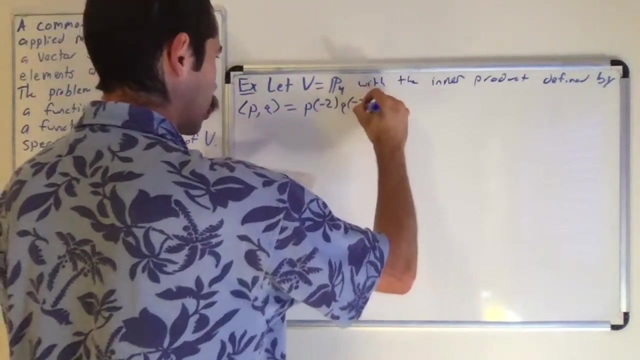 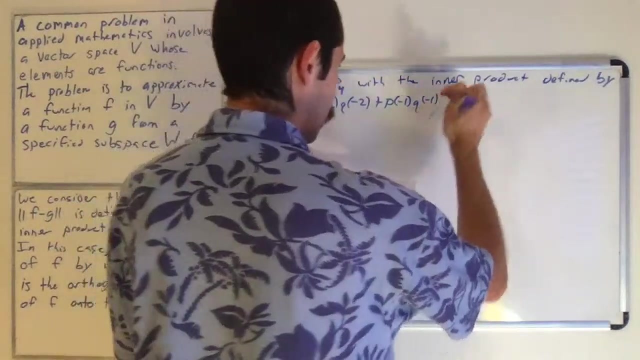 OK, so we'll start by saying: let V equal P4.. We're going to need some more space. So, with the inner product defined by, PQ is equal to P of negative 2, Q of negative 2, plus P of negative 1, Q of negative 1, plus P of 0, Q of 0, plus P of 1,. 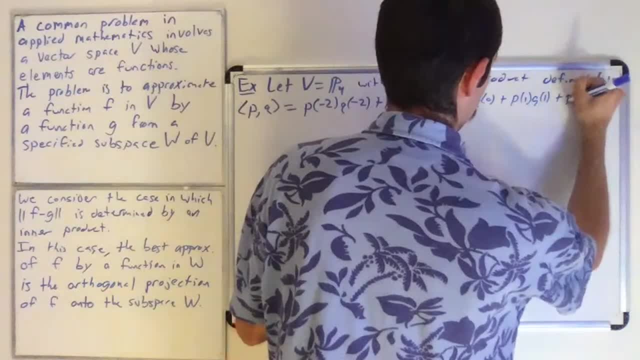 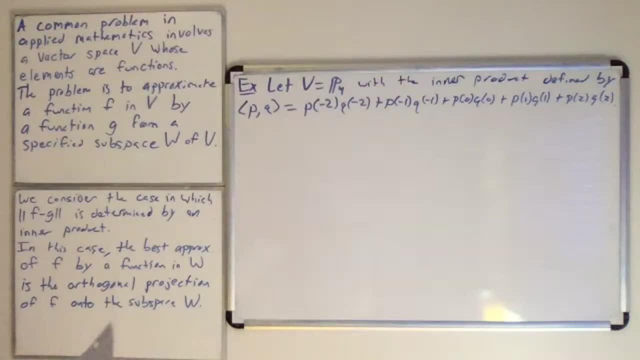 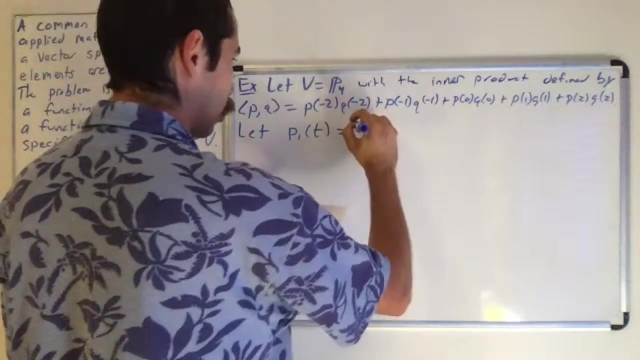 Q of 1.. OK, so that's our inner product. We've got to evaluate our polynomials at negative 2, negative 1,, 0,, 1, and 2, and multiply them together like this. So we'll let P1 of t equal the polynomial 1, right. 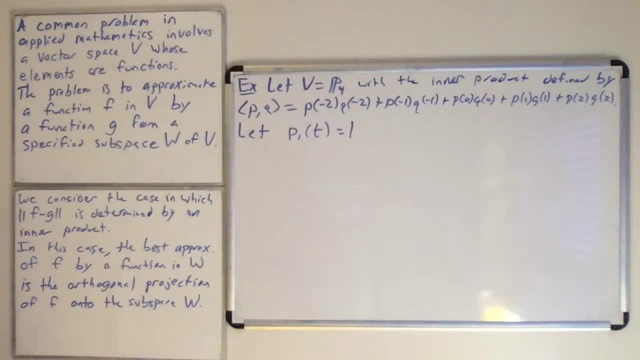 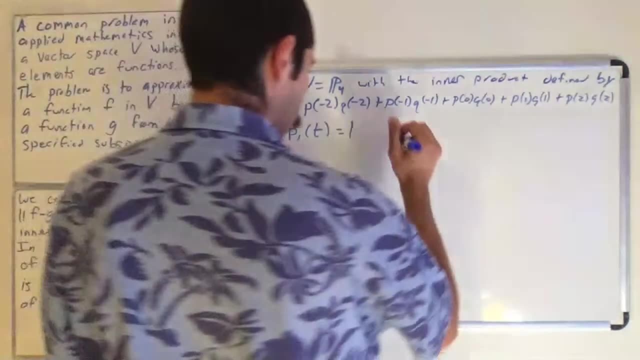 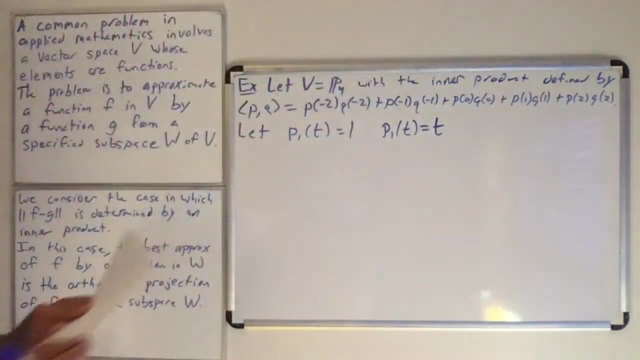 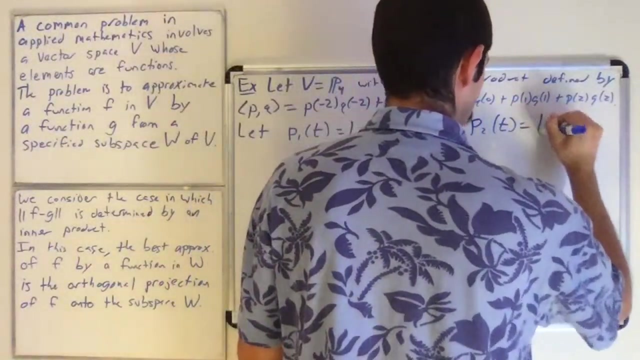 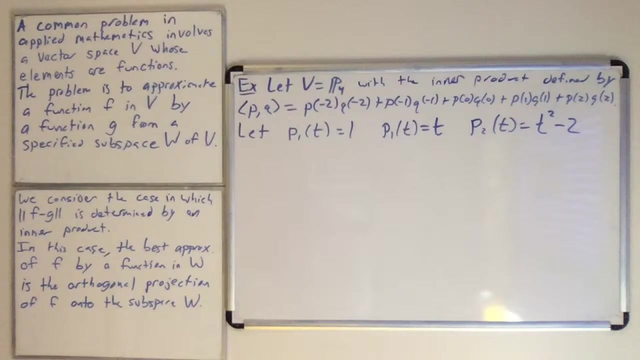 This is in P4, because its degree is 0. And P4 is polynomials of degree, at most 4.. We'll let P1 of t equal t And we'll let P2 of t equal t, squared minus 2.. OK. 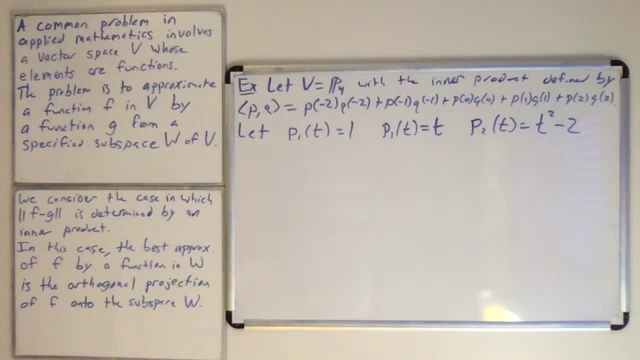 And so the question is: Show that, OK, P1,. let's make sure we get this right. this is P0.. I'm not sure why I labeled them like this. All right, P0 is 1, P1 of t is t and P2 of t is t squared minus 2.. 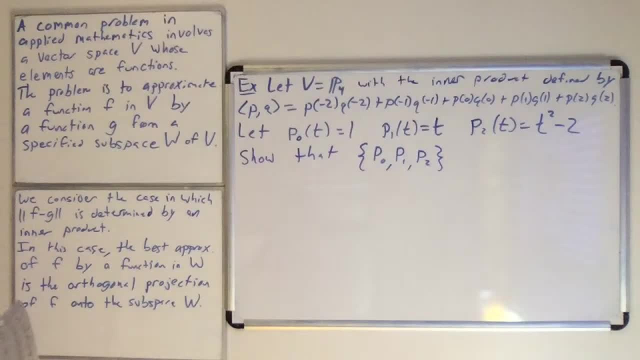 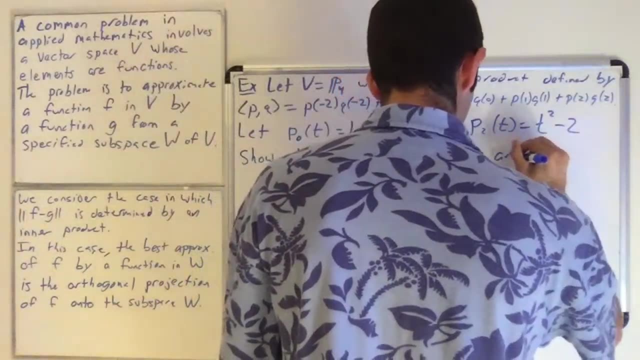 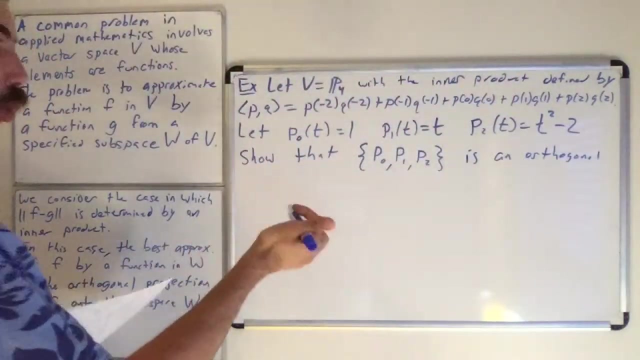 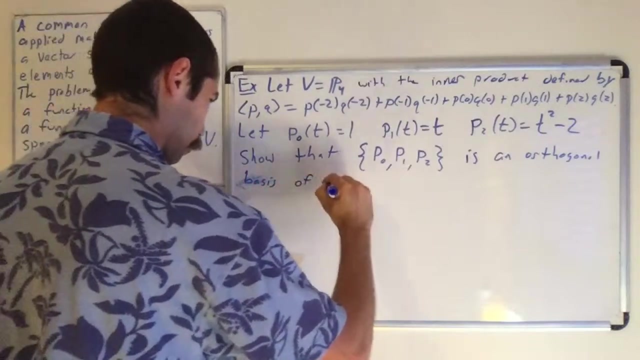 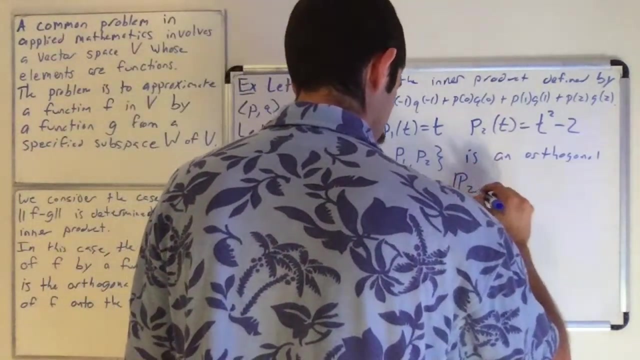 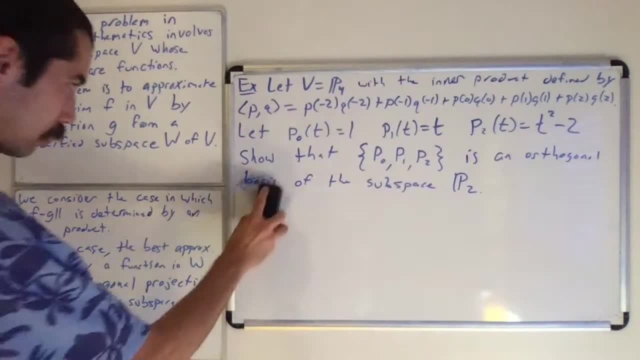 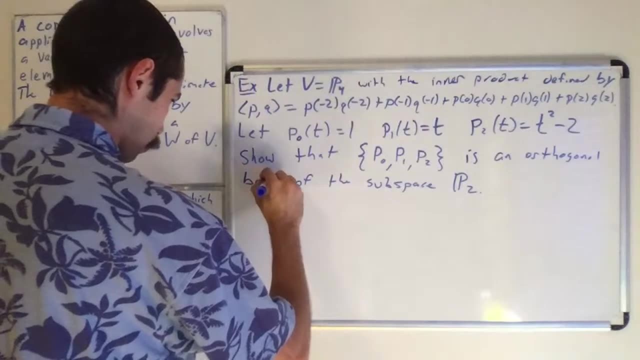 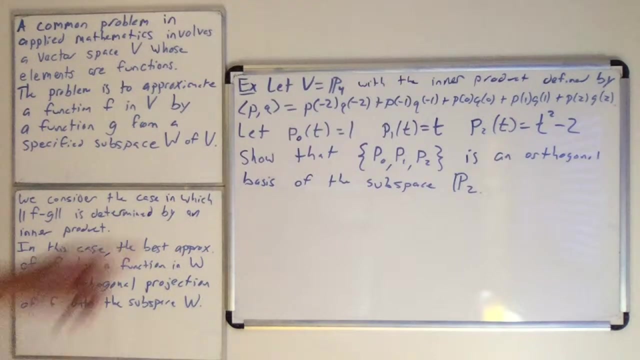 I'm not going to write the second part yet. All right, So we have these three polynomials. How do we show that? so this is for the chat. how do we show that P0,, P1, and P2 is an orthogonal set? 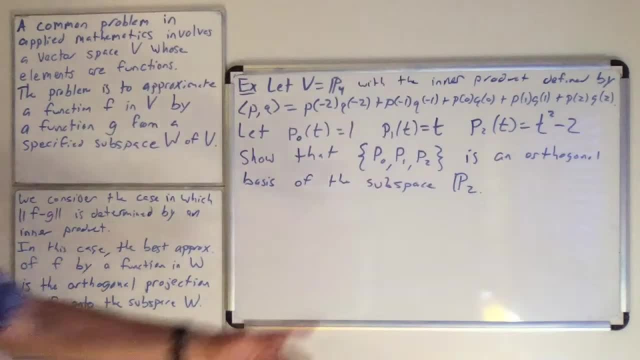 All right, an orthogonal set. right, because we need to show it's an orthogonal set that spans all of p2, to show it's a basis. so how do we show it's an orthogonal set with respect to this inner product? so yeah, that's right, taylor. so we want to evaluate the inner product of p0 and p1. 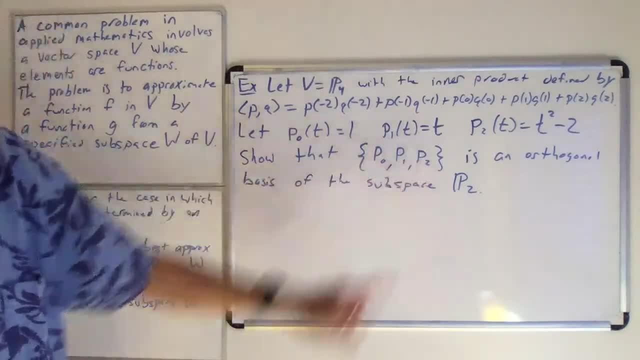 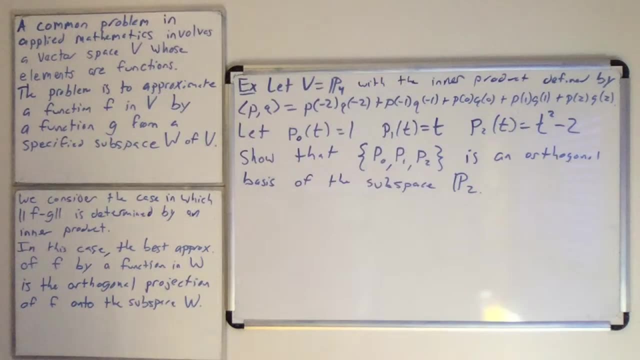 and let's hope we get zero. let's take the inner product of p0 and p2, and we should get zero, and then the inner product of p1 and p2, and again we should get zero. okay, and then the question is so, once you show that, then the question is: how do we know that? 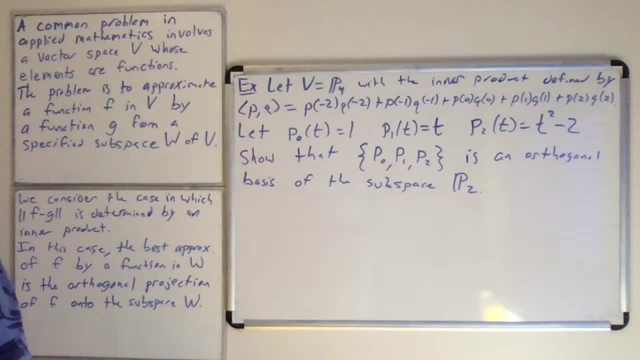 this is a basis of p2. sorry the span. how do we know that the span of this set is, uh, is p2, or how do we know that this set is a basis for p2? all right, you, okay. would anybody like a little bit more time to uh work on this, or are we good for me to? 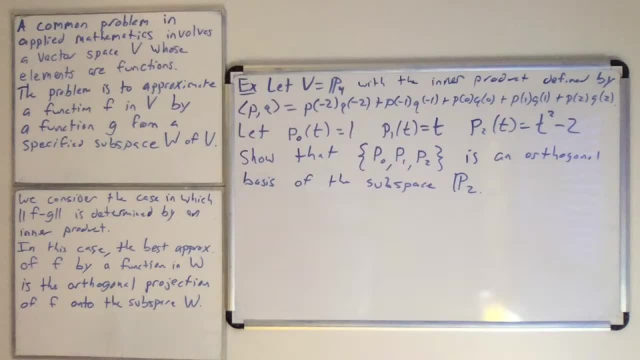 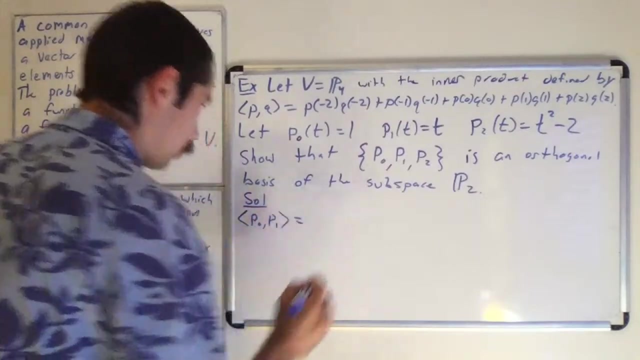 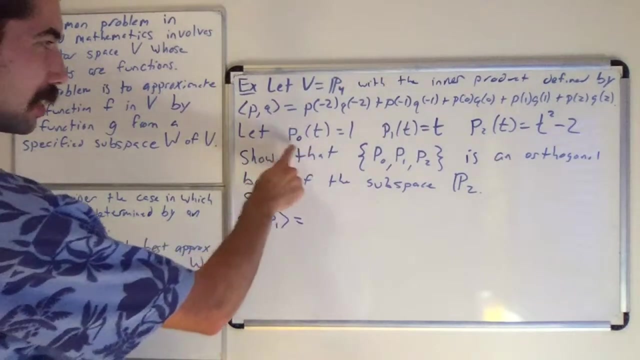 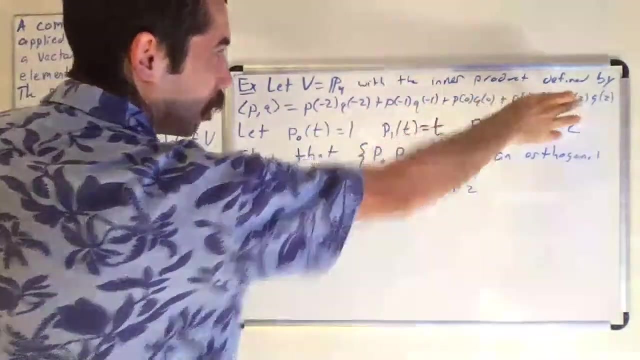 to get started. i'm fine giving more time if you need. it all right, i'll start working this through. let's start with p0 times p1. so p0 is always one. so all these terms in our inner product that come from the first term is just one, one, one, one one. 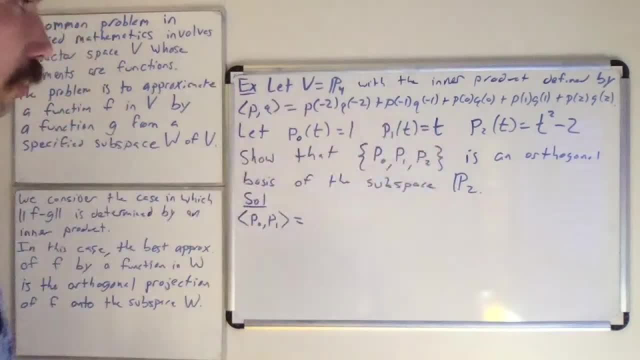 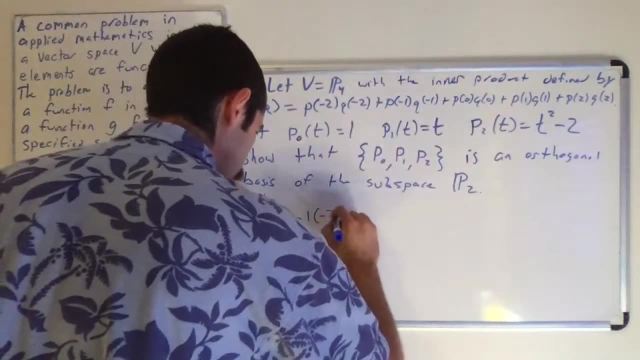 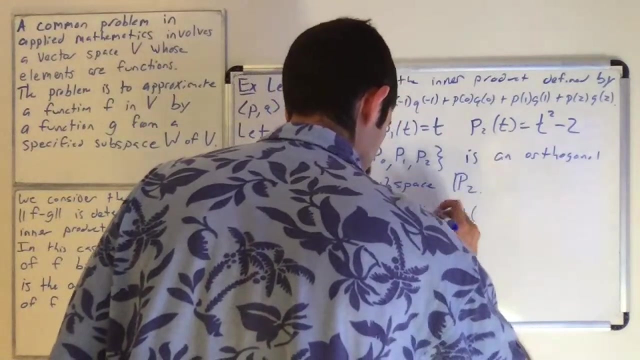 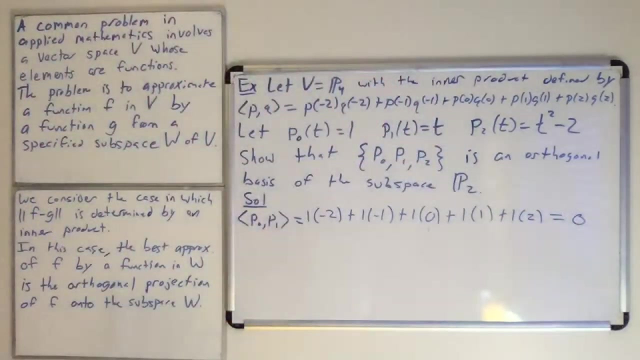 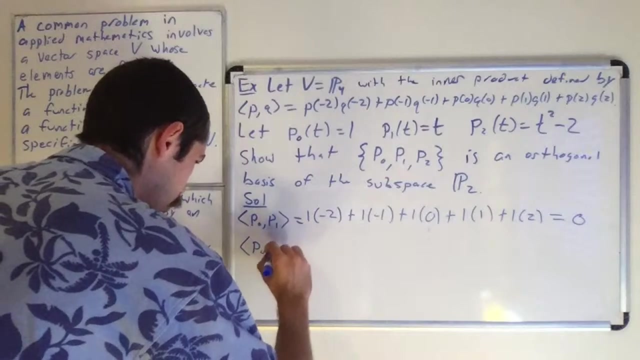 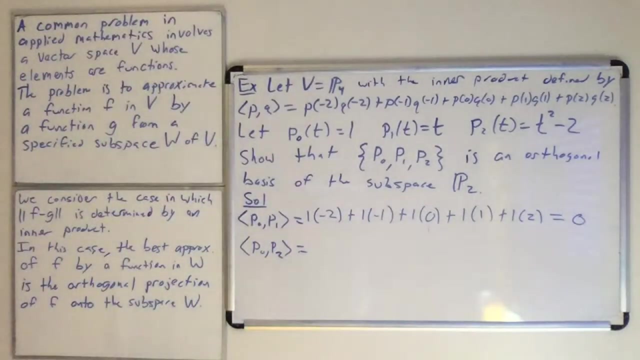 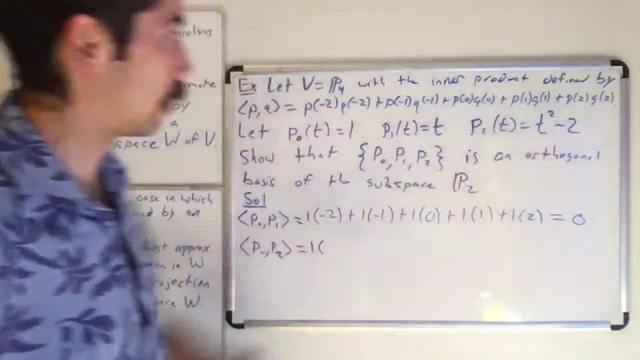 and p1 is the, is the uh polynomial t. so it'd just be negative two, negative one, zero one and two. so and when you add all those up you get zero. okay, now we'll do p0 times p2: t squared minus two, evaluated at negative two, uh is two. 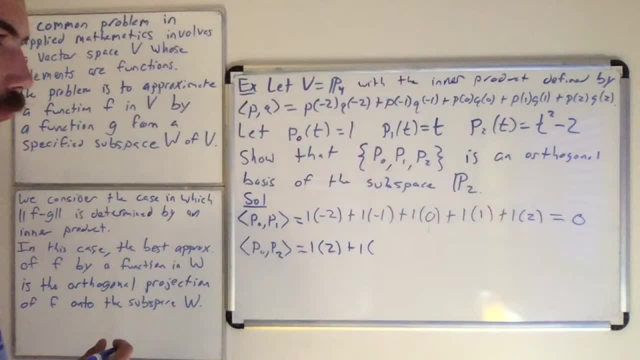 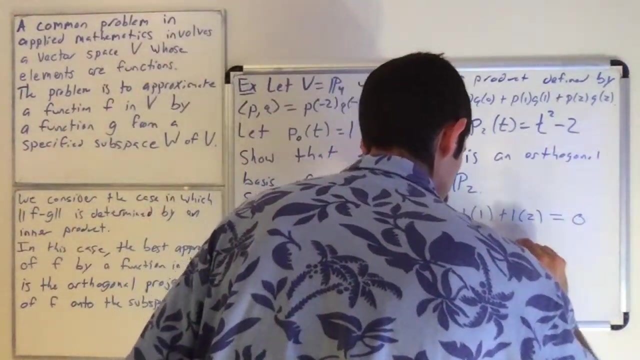 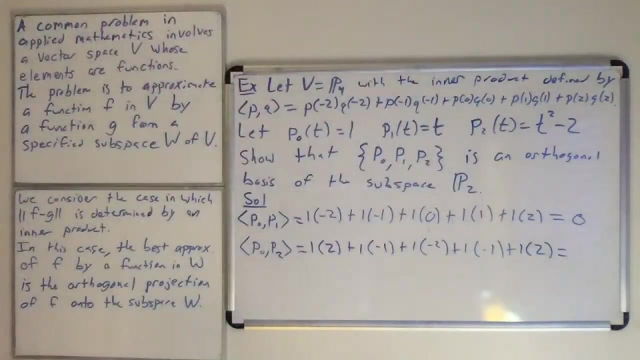 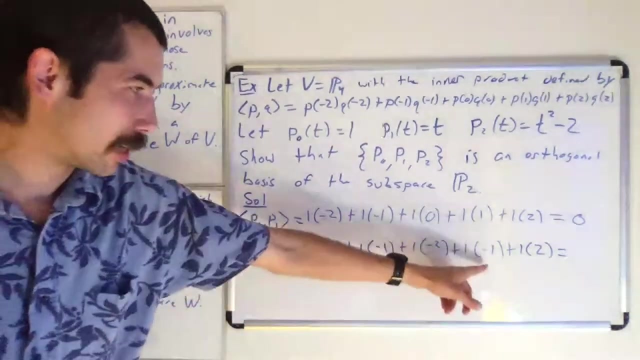 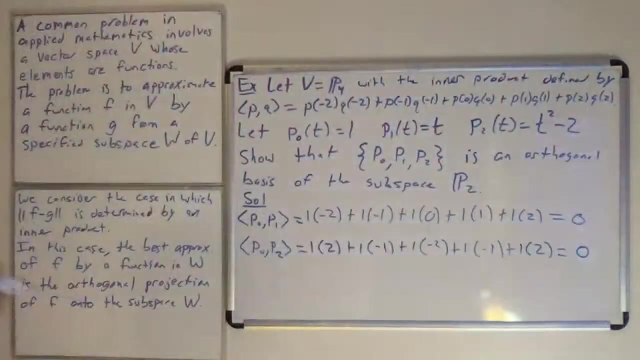 t squared minus two, evaluated at negative one, is negative one. t squared minus two, evaluated at zero, is negative two. this is a even function, so it works out to be this: two minus one minus two minus one plus two, that's zero. so, and then p1 times p2. 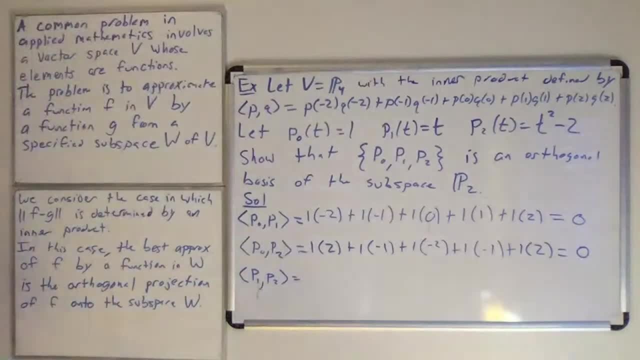 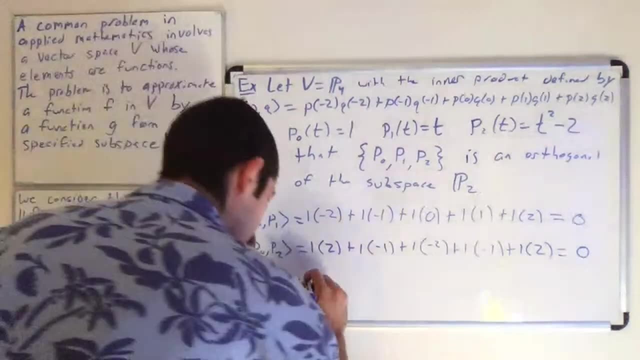 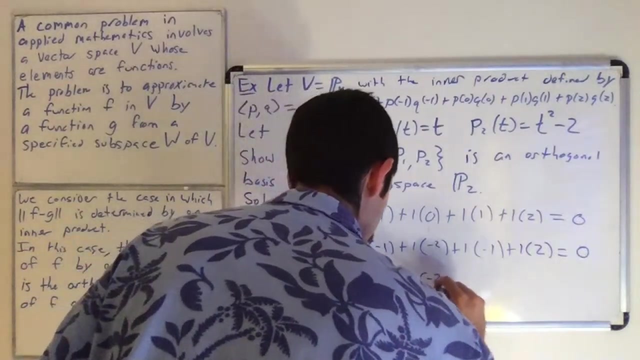 well, this is p1 evaluated at negative 2 and this is p2 evaluated at negative 2, so it's negative 2 times 2 plus negative, 1 times negative, 1 plus 0 times negative, 2 plus 1 times negative, 1 plus 2. 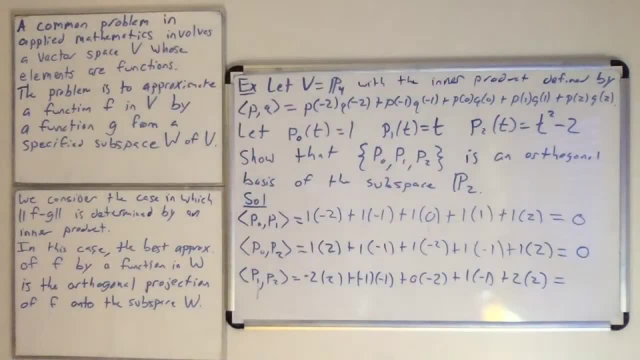 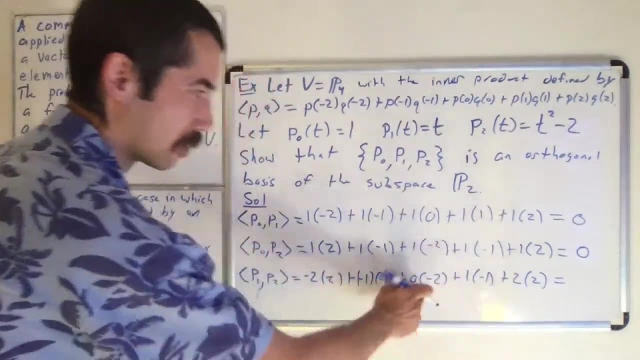 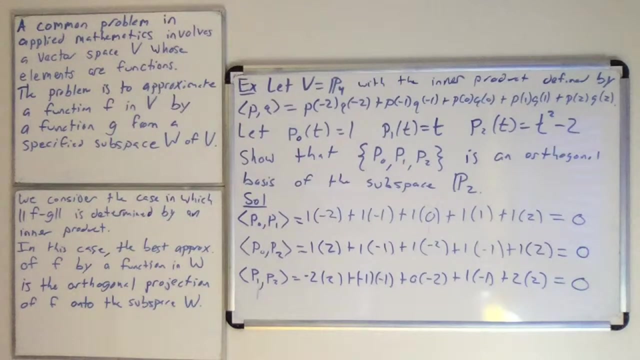 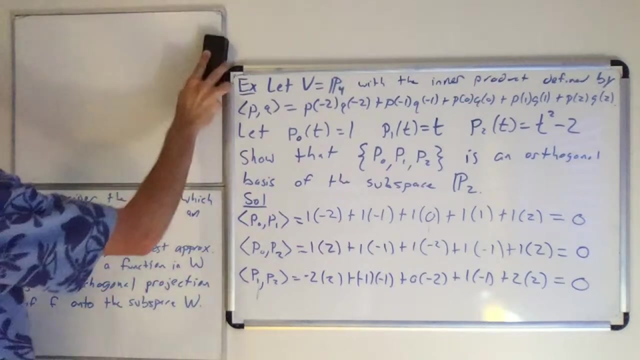 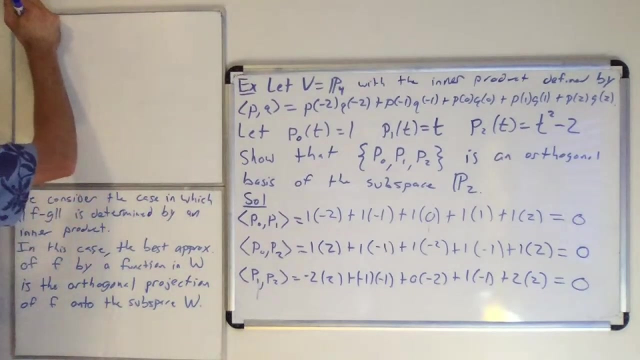 times 2 negative, 4 plus 4 cancels, 1 minus 1 cancels and that's 0. so this is all 0. okay, so we showed it's an orthogonal set. how do we know? it's a basis for p2. it's linearly independent, that's true, but, like, for instance, p0 and p1 is also linearly independent. 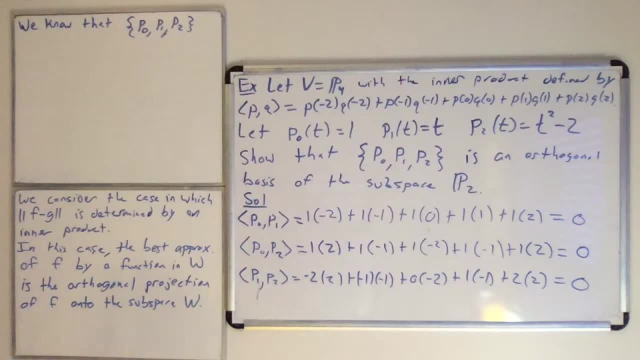 so what else? well, maybe it's. maybe you'd have to look back in your notes a little. it's that there's three of them, right, and the dimension of p2 is three. so any three linearly independent polynomials in p2 are independent polynomials in p2 and p2 is independent polynomials in p2. 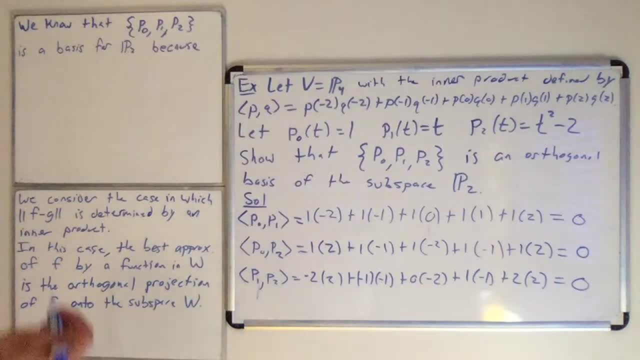 span p2. sorry, it's a basis for p2. so we know that p0, p1, p2 is a basis for p2 because any three linearly independent and p2 so because any three linear in the linearly independent polynomials in p2 is a basis for p2. 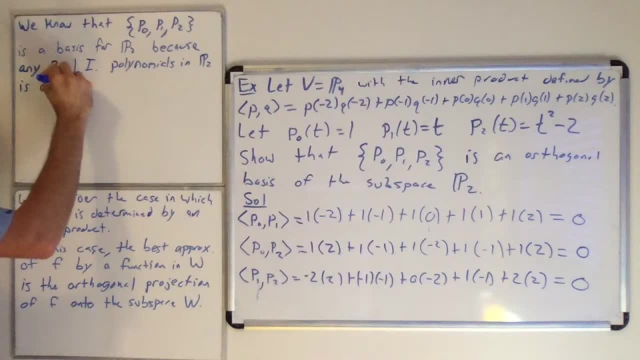 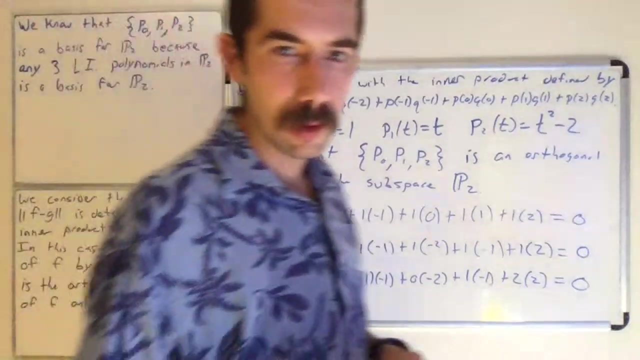 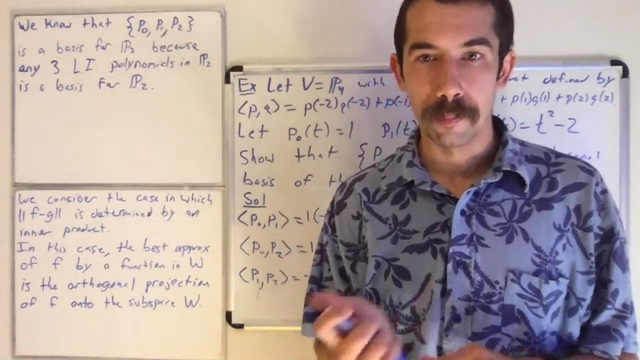 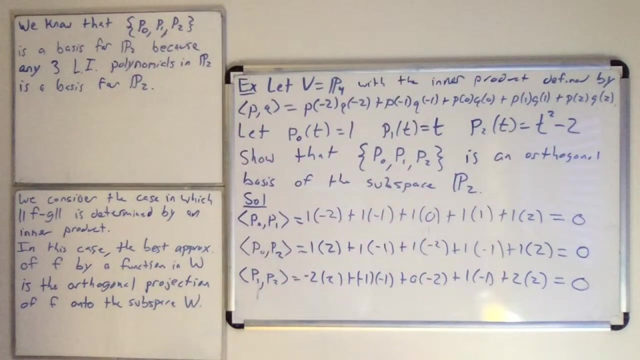 right, and that's because of the dimension, the dimension of right. p2. we said that p2 and r3 are basically the same vector space, so their dimension is three um. so yes, so since we showed that, since we showed we had an orthogonal set, we had a theorem that said all orthogonal sets are linearly independent. 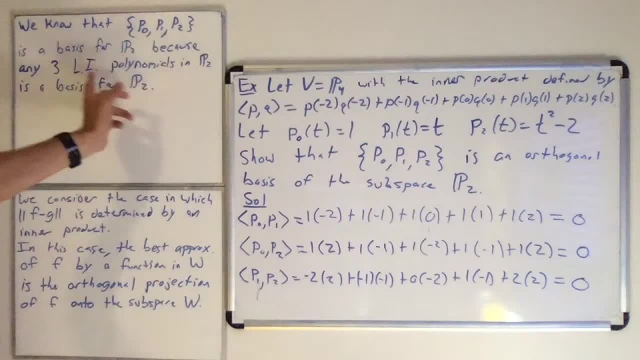 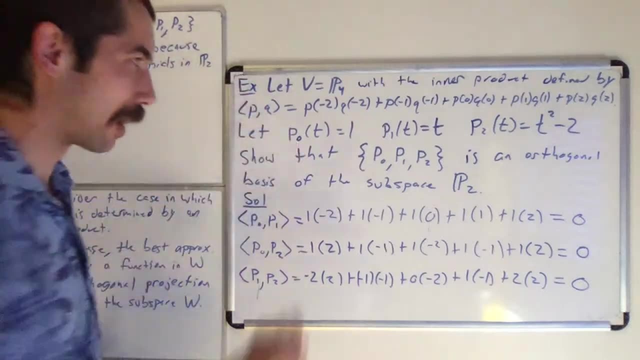 and since there's three of them, it must be a basis for p2, right, and that's because- and you know, we also have to be careful- we have to make sure that each of these live inside of p2 and they do right. p, this polynomial, has degree two, this one has degree. 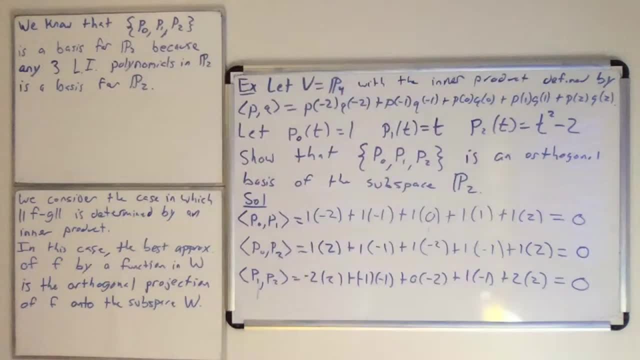 one, and this is degree zero. okay, so that's the first part of the question. so now that we have an orthogonal set, it makes sense to do an orthogonal projection. so find the best approximation to the polynomial. so find the best approximation for the polynomial five minus one half t to the fourth power of p. 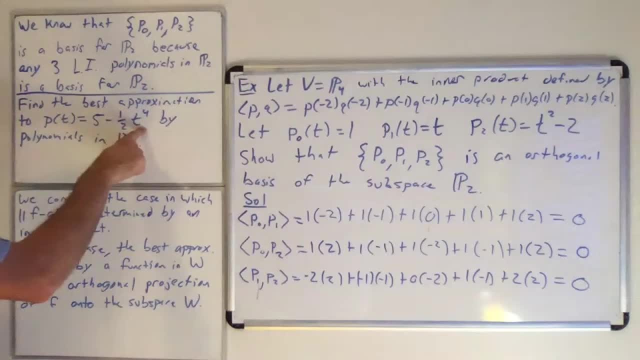 okay, so this is a degree four polynomial and we want to approximate it by degree two polynomials. okay, so how are we going to? how are? how are we going to do this? okay, so how are we going to? how are we going to do this now? all right. 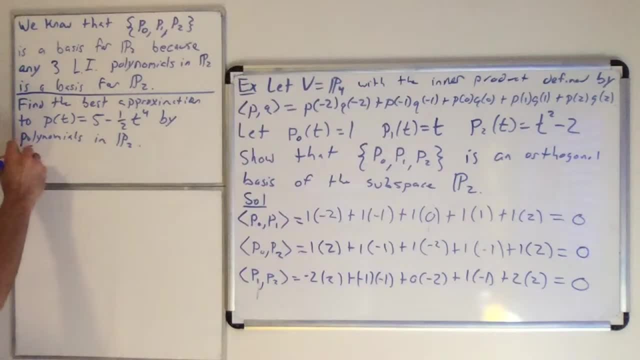 all right. so so you, yeah, you're on the right track. chow, we want to not find the least square solution, but we just want to find the orthogonal uh projection. so it's the same idea. the least square solution would tell us, like the coefficients of of p0, p1 and p2. 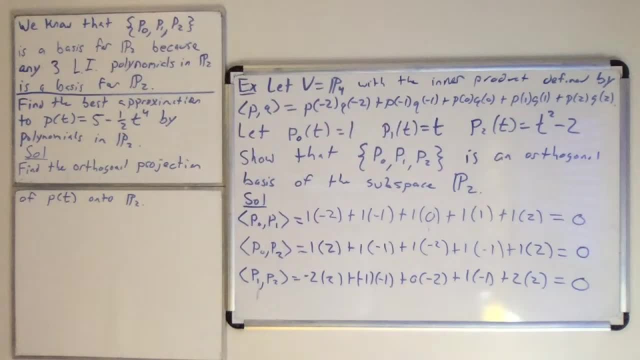 which. that's one way to solve it, but we could just find the orthogonal projection, so we'll call that p hat, and the way we get the orthogonal projection is exactly the same as how we did it with column vectors. it's p times p0, over p0 times p0 times the polynomial p0. 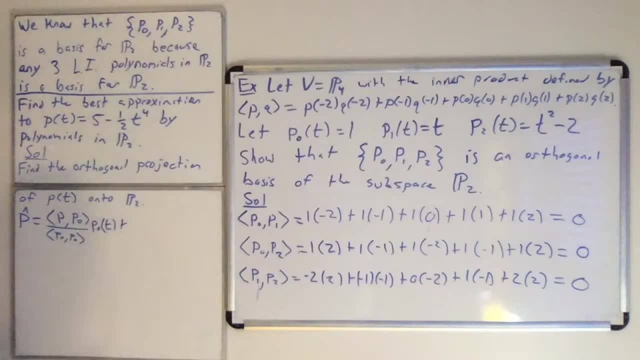 and we get the orthogonal projection, which is exactly the same as how we did it with column vectors. it's p times p0 plus p times p1, over p1 times p1 times the polynomial p1 plus p times p2 plus p times p2. 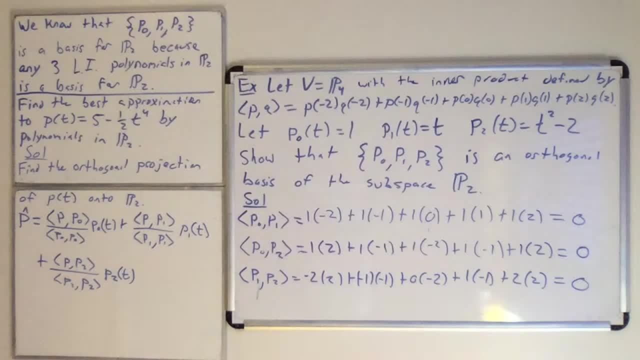 over p2 times p2 times the polynomial p2. okay, and so when we work this out, when we work this out, this polynomial, this, you know it's going to end up with a degree two polynomial. maybe it's less than two will be. we'll have uh. 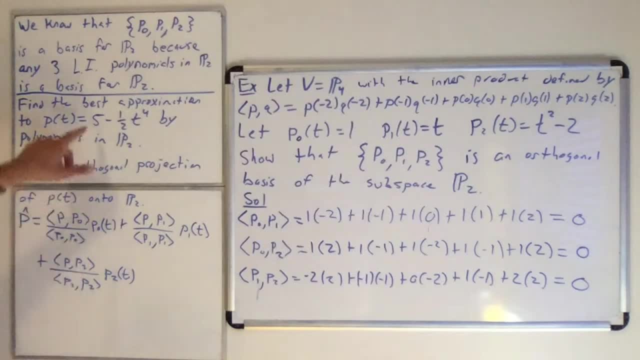 it will be as close as possible to this um, to this degree four polynomial, using this inner product. okay, so i'll give you a few minutes to try to work out these calculations, and then we could do it together- and when I say together, I mean I will just do it and you guys will watch. 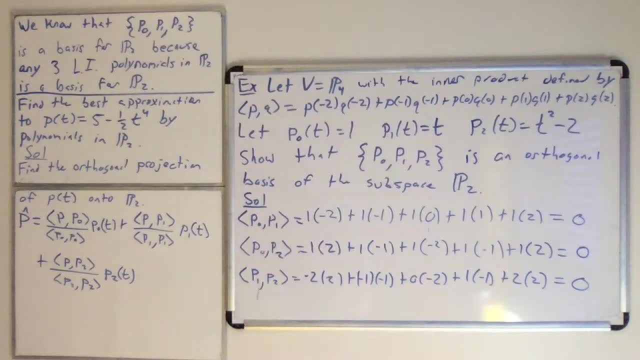 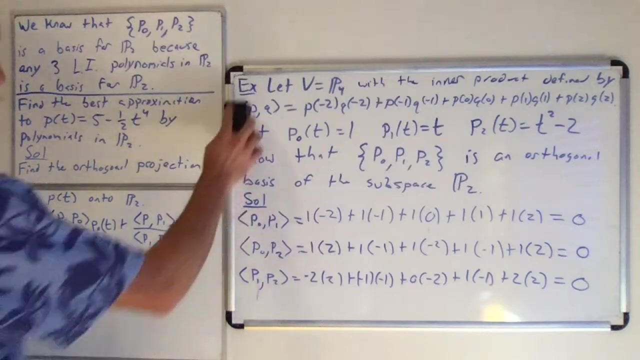 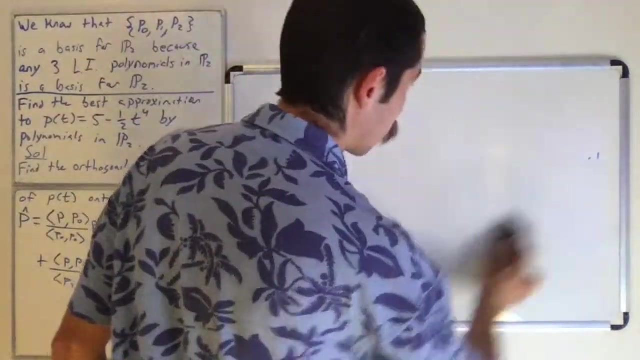 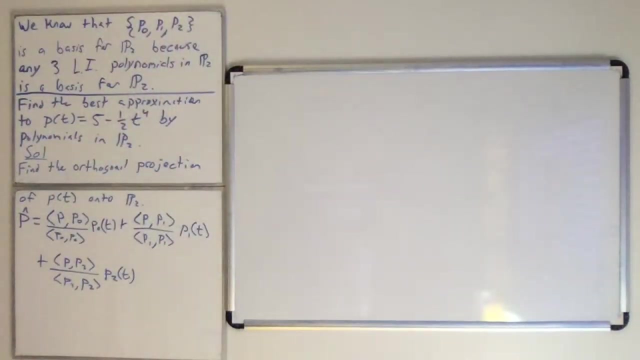 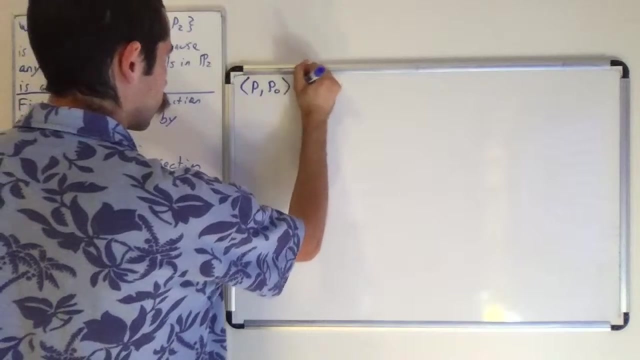 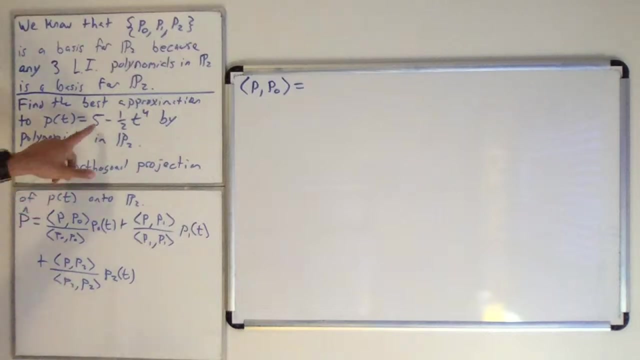 please ask any questions if you need something to be clarified. you all right. so we need to find p times p0, p times p1, p times p2 and then each of the basis vectors times itself. so I'll just work out these calculations. so we evaluate our polynomial at negative two. 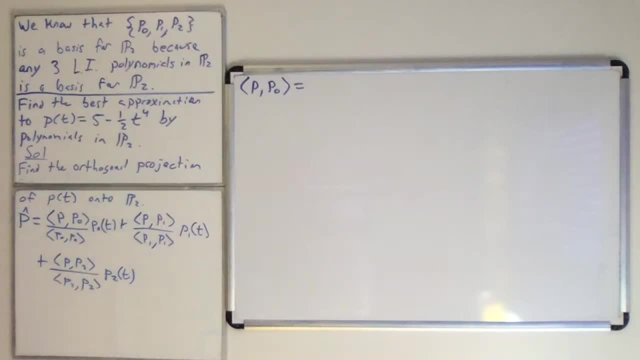 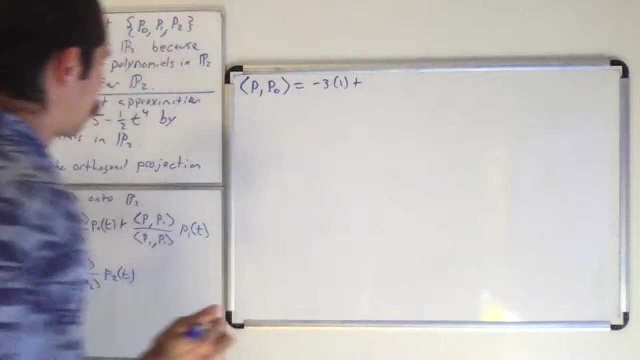 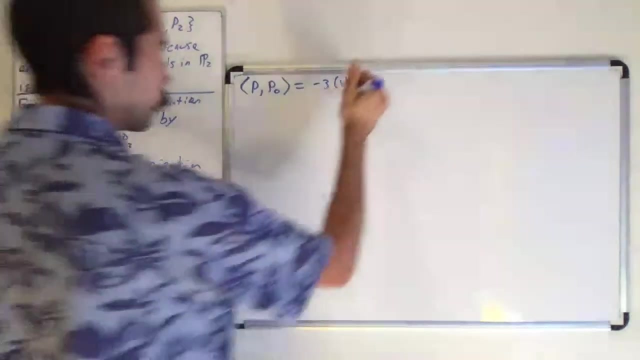 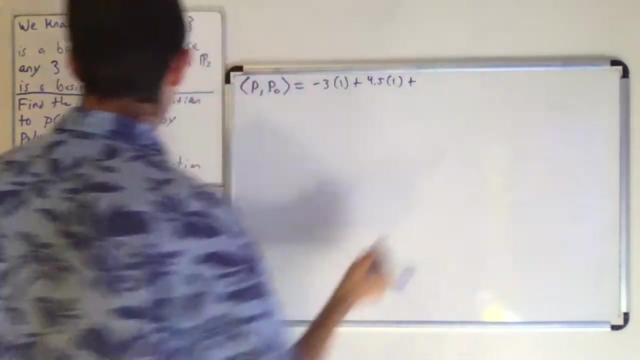 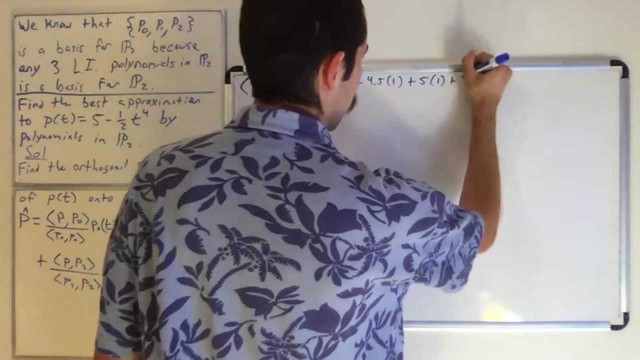 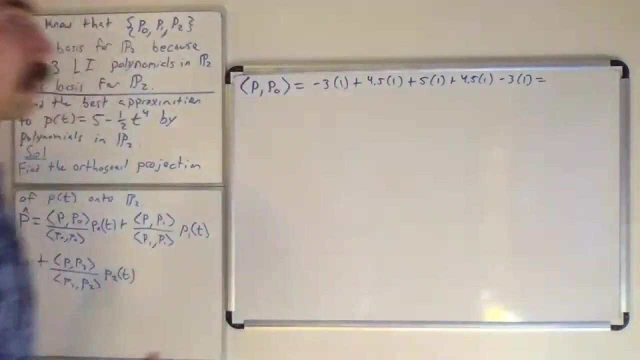 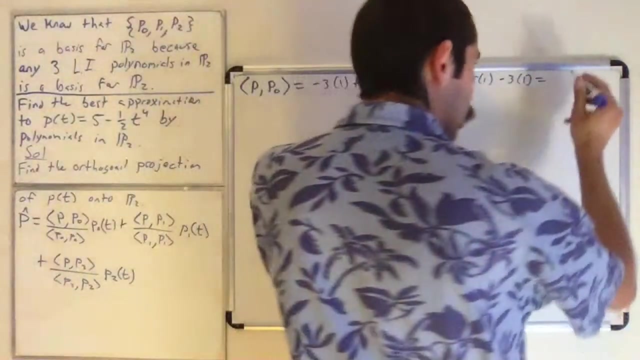 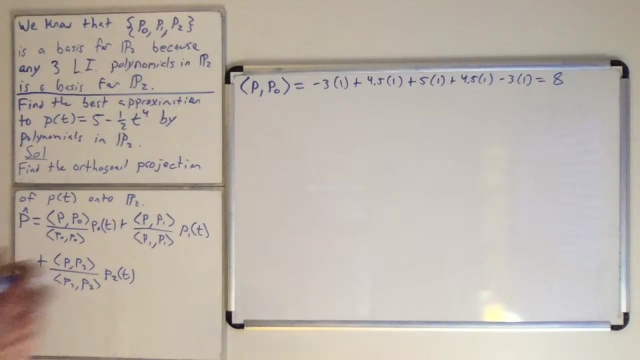 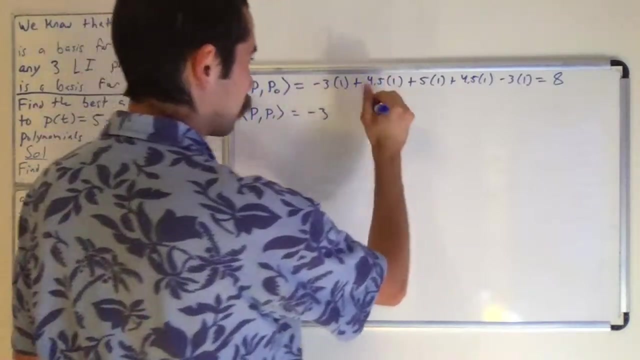 we evaluate it at negative one, we evaluate it at zero, we evaluate it at positive one and a positive two, and add all of them up and you get 14 minus 6 is 8, all right, so so these coefficients are going to be the same for all of them. 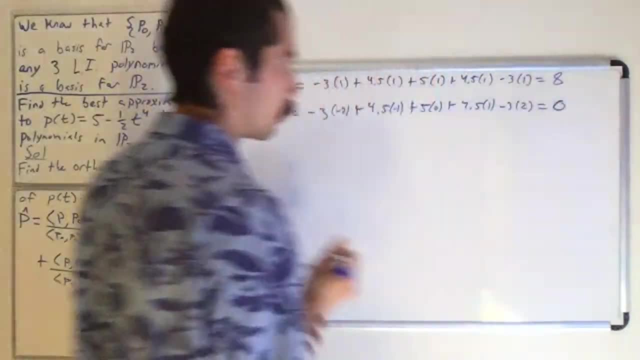 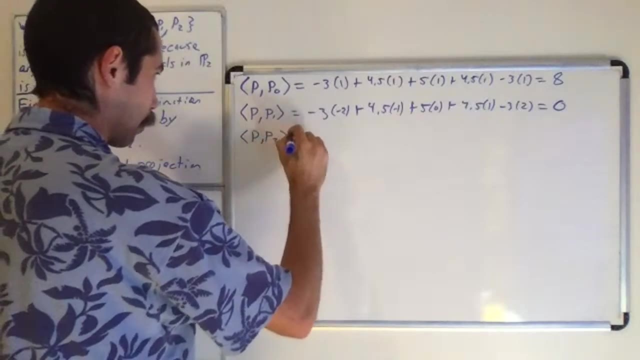 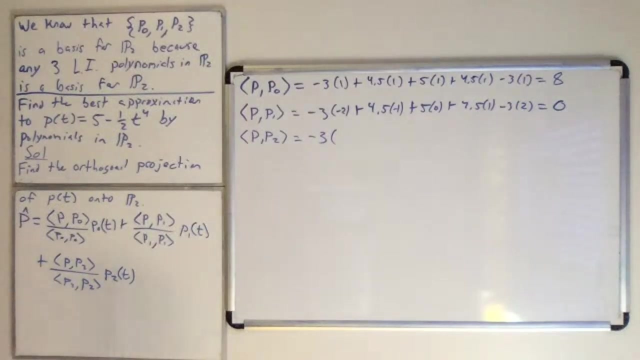 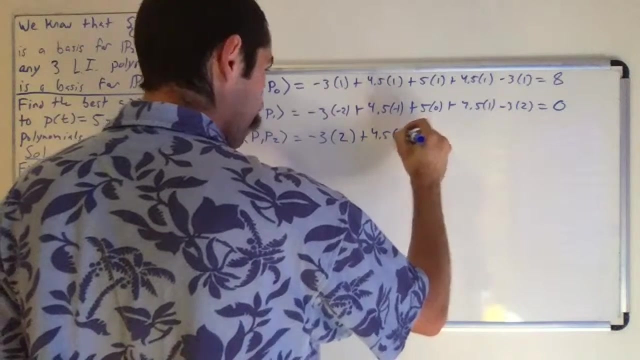 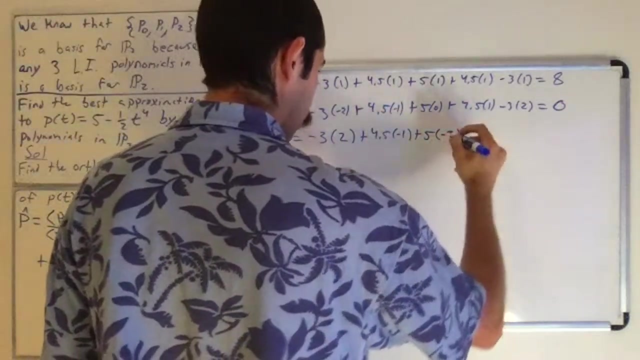 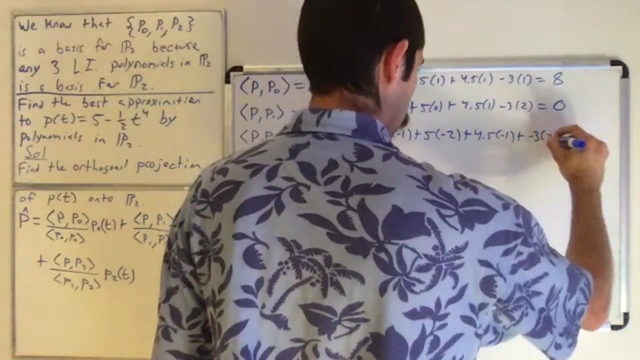 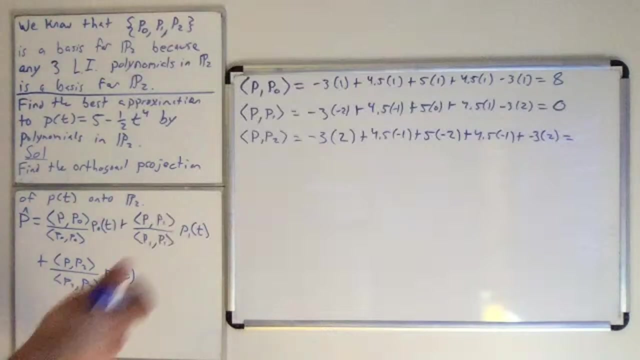 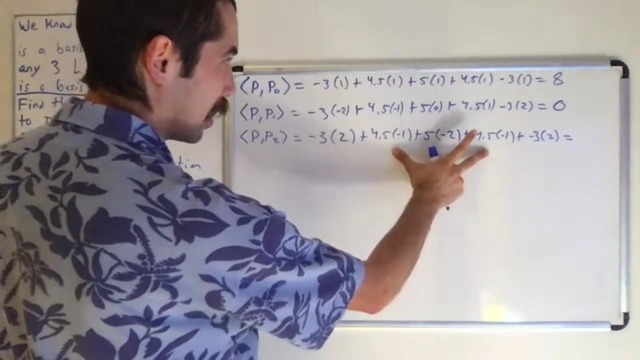 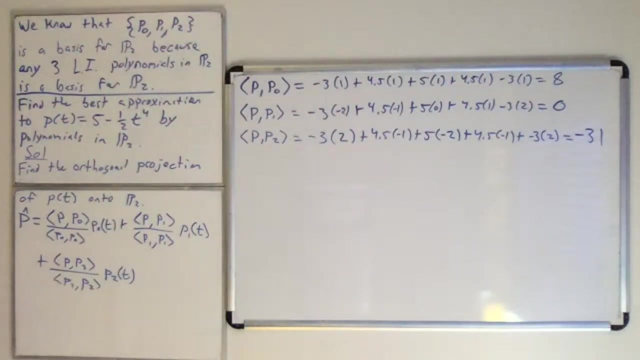 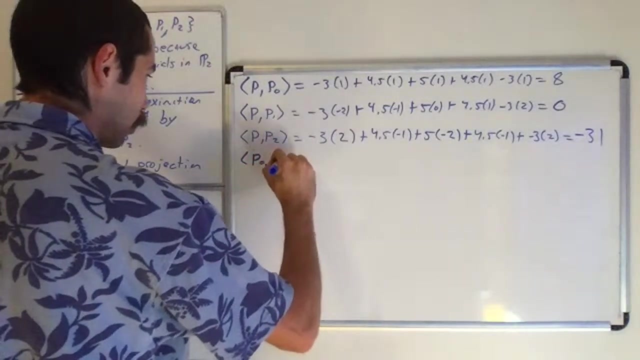 so and so and so and so when you add these up, you get zero. all right, when you work all this out, you get: let's see, negative six minus nine. uh, negative 31. you get. is that true? yeah, so negative 12 minus nine minus ten. okay, so now we have to compute p zero times itself. 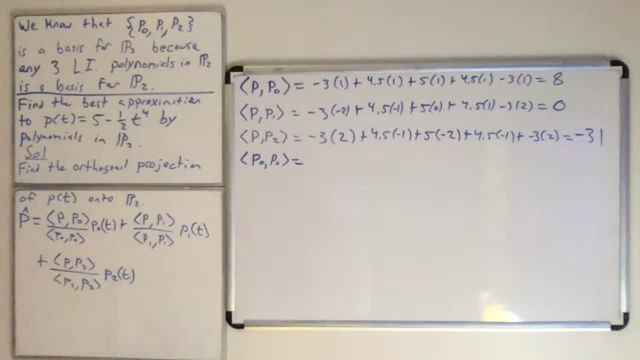 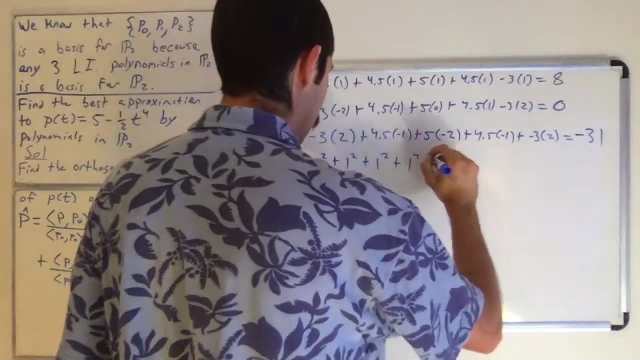 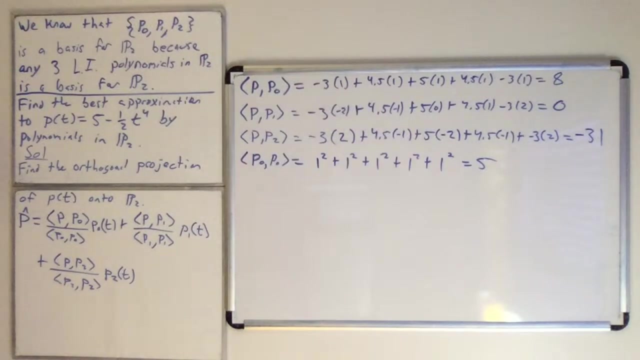 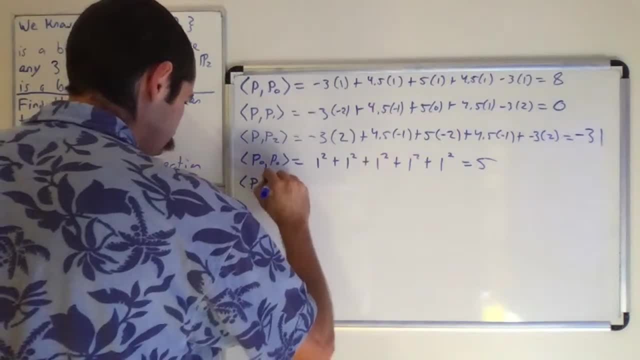 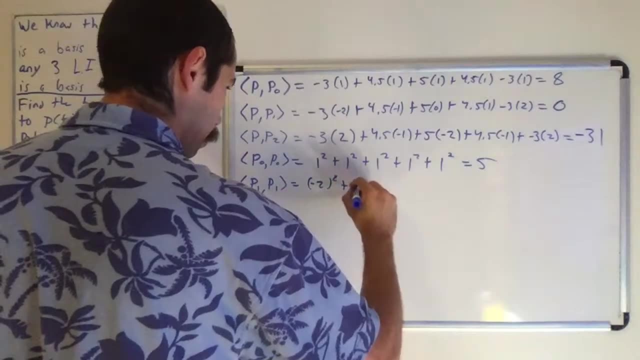 which we could expect it will work, so that you know, we could possibly start to learn it. three by one. they're ethered out, every single element. we're using a rule called the p one, so i'm going to drag in thetrehod by two. 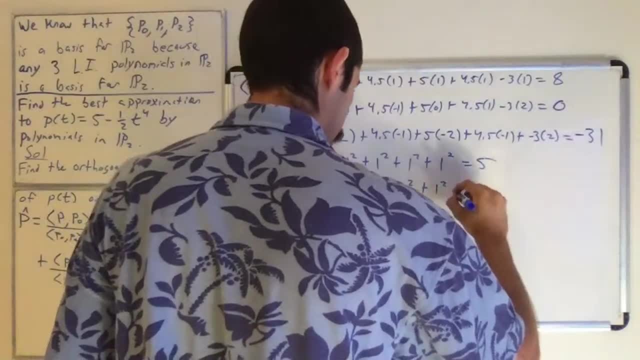 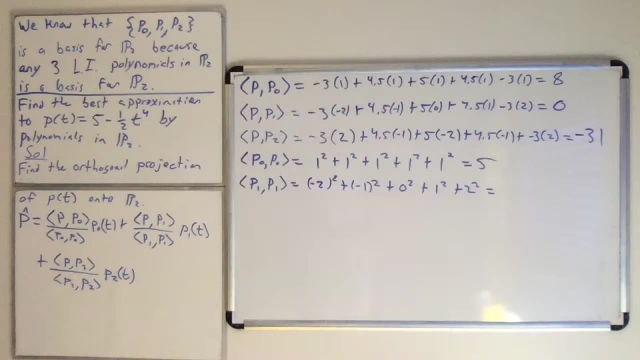 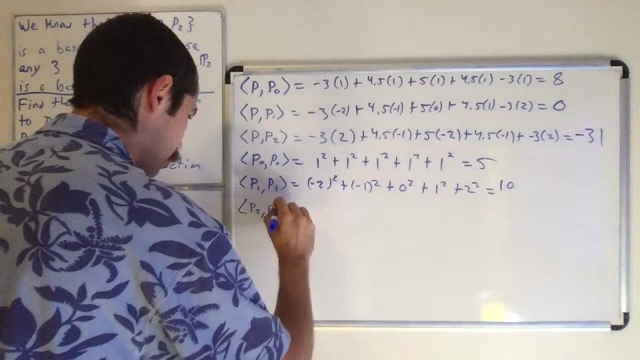 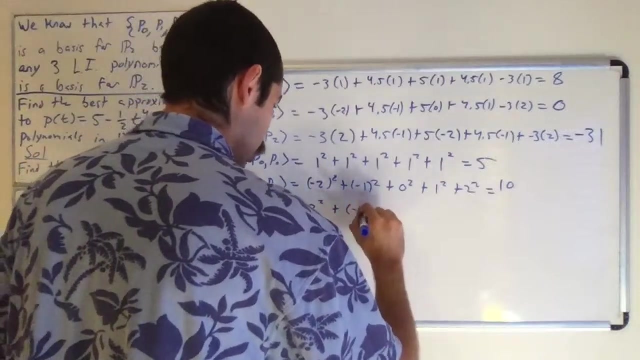 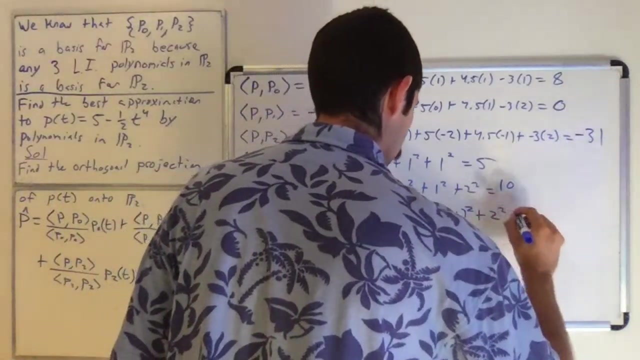 of the operators, and so we have length allowed and payload allowed, Pause주 r plus 1 plus 0 plus 1 plus 4, that's 10, and then p2 times itself is 2 squared plus negative 1 squared plus negative 2 squared plus negative 1 squared plus 2 squared, which. 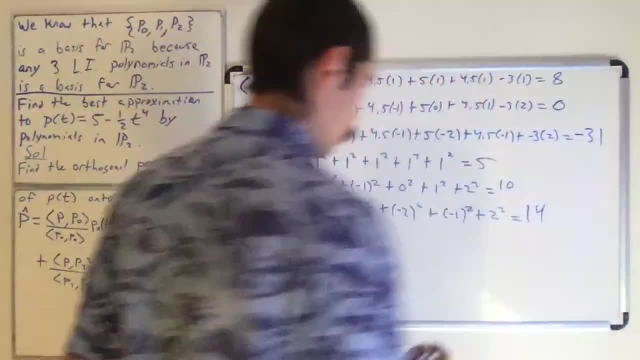 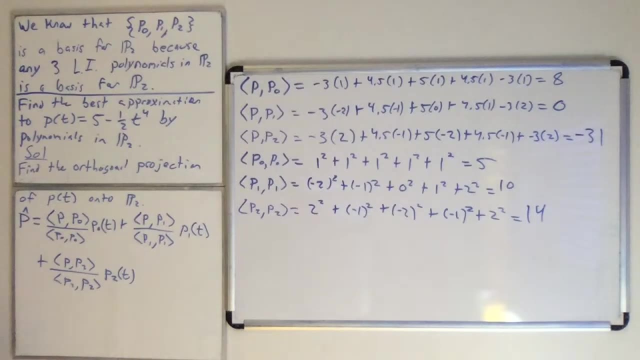 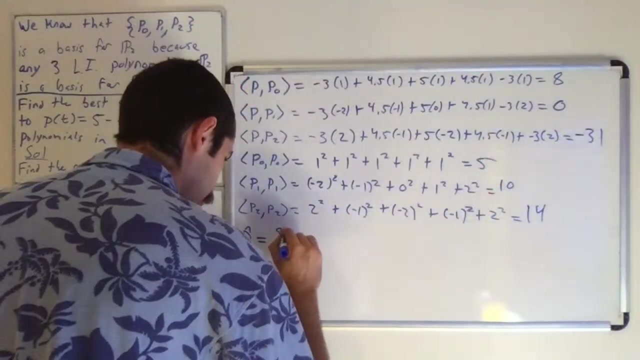 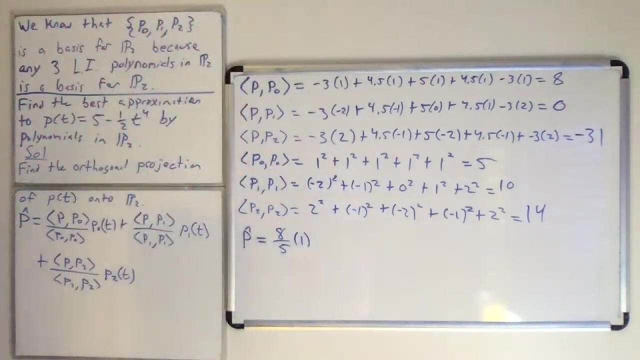 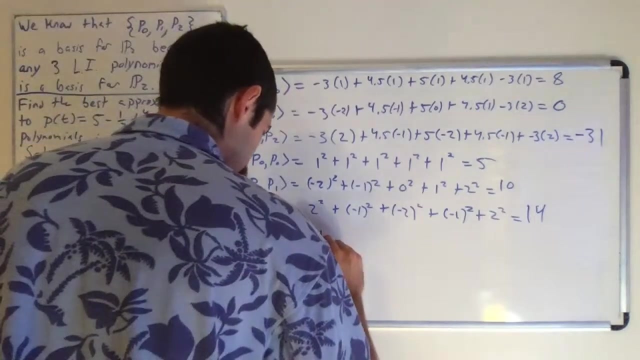 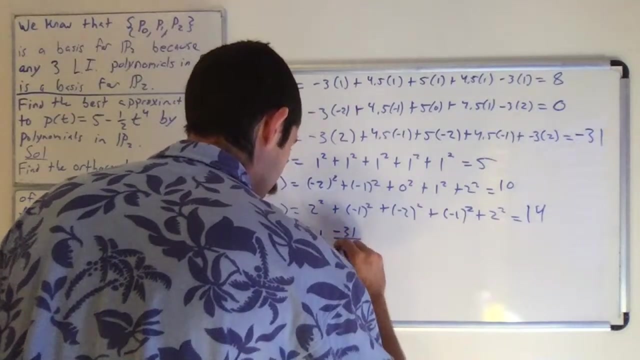 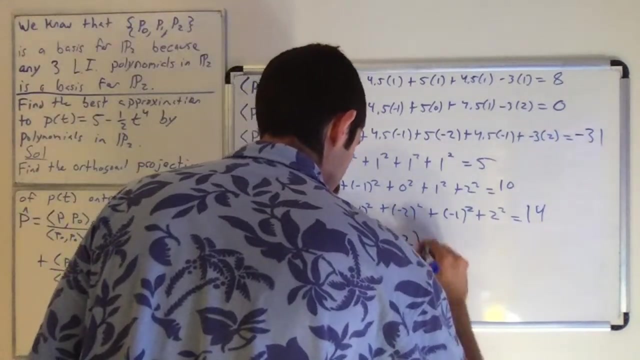 is 14.. Okay, so we did it. Our approximation, which we can call p hat, is equal to 8 fifths times p0,, which is the polynomial 1. Plus 0 tenths p1, plus negative 31 fourteenths times the polynomial t squared minus 2.. 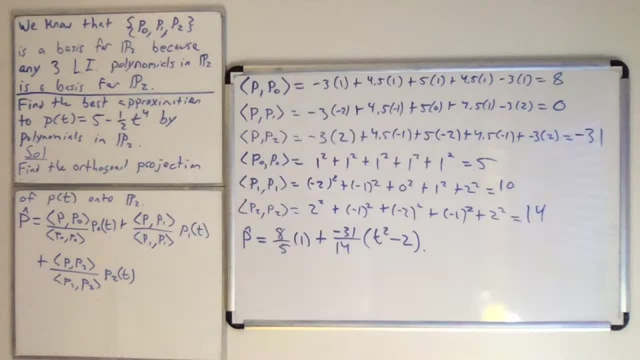 Okay, so this polynomial is closest, in the sense of this inner product, to this polynomial 5 minus 1 half t to the fourth. So this is the closest degree 2 polynomial to this degree 4 polynomial in the sense of this inner product. 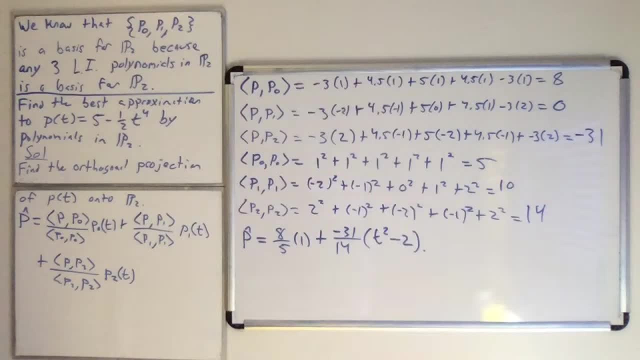 Okay. Okay, I know this question had a lot of competition to it, but this is identical to what we've been doing last week. this idea of orthogonal projection: Just because we have a different vector space and a different inner product doesn't mean. 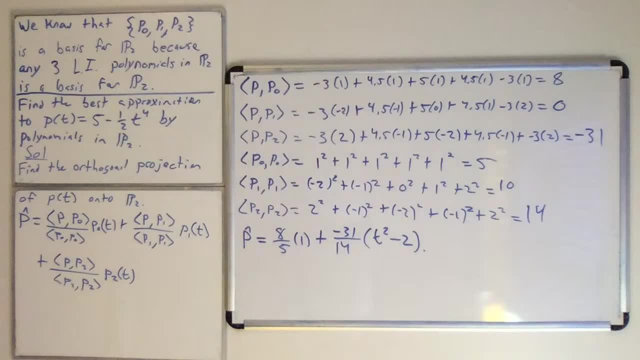 our concepts of orthogonal projection don't work anymore. Does anybody have any thoughts or feelings that they would like to share with the class about this question? You know it could be as simple as a thumbs up or a thumbs down. Taylor's happy with the question. 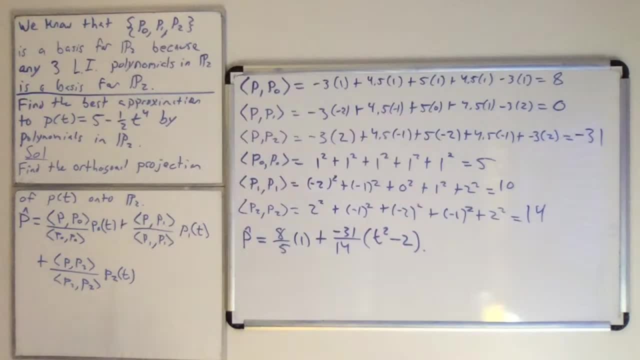 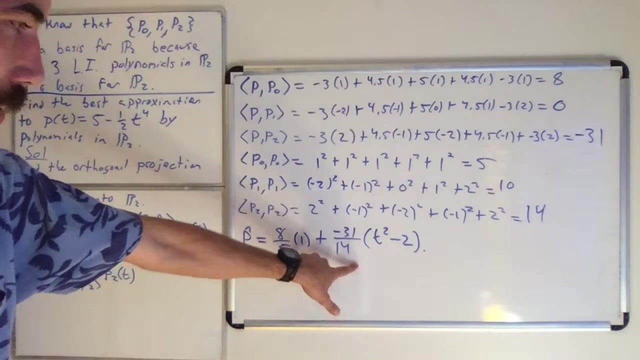 That's good to see. All right, We could. I mean, I can't do it now because we're using a webcam, but we could plot this with Desmos and you could see that it's going to have similar shape to 5 minus 1 half t. 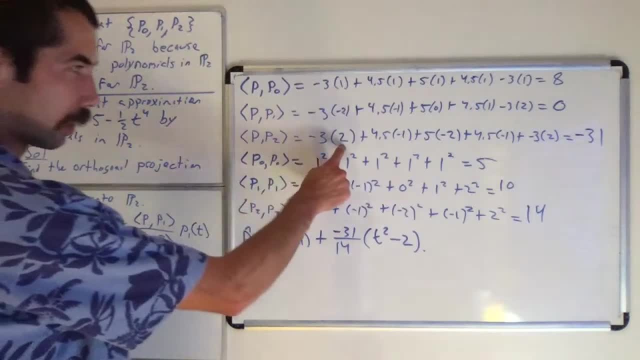 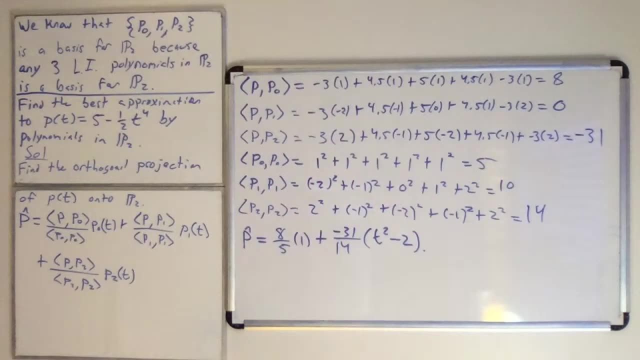 squared And in fact it's going to be closest when we're at the values 2, negative, 1, negative- sorry, negative 2, negative, 1, 0.. Nice cruise 1 and 2.. So at those five values that we evaluate our function at, you know it's going to be a 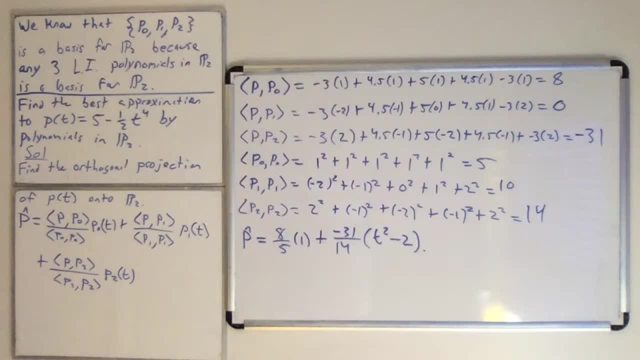 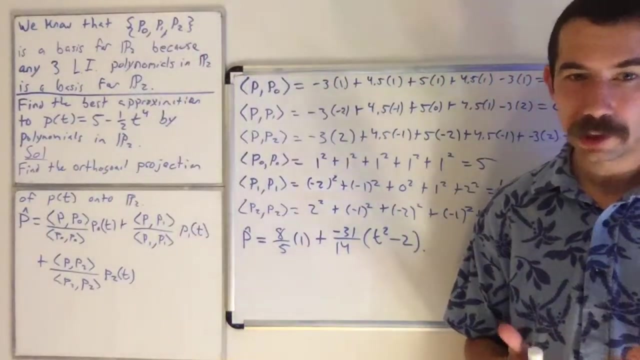 pretty good match, Okay, Well, I think this is a good place to stop for today. Tomorrow, tomorrow, we'll start class Um with a couple of with a couple of proofs. So if you like proofs, that's great. 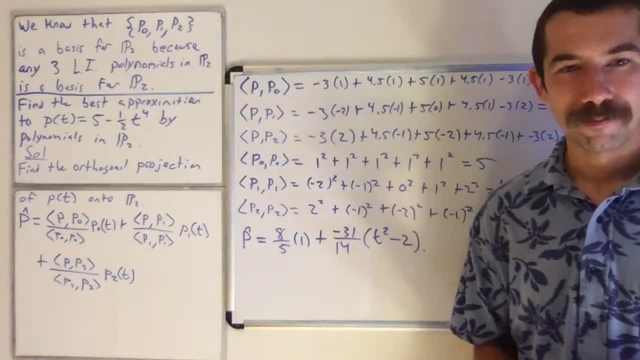 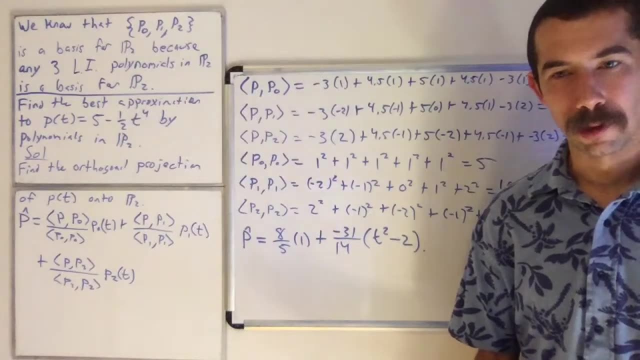 We'll get some practice with those. Um, if you don't like proofs, well, maybe you'll like them after class tomorrow, because they're, they're, they're neat. Um, these ones are going to do All right, So make sure to hit the like button before you get out of here. 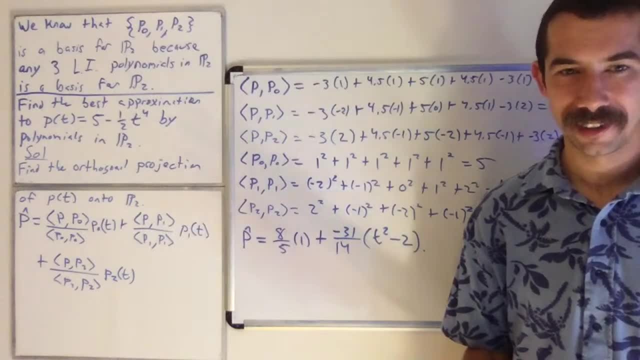 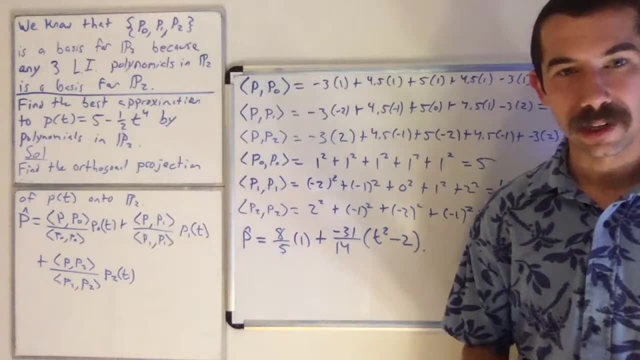 As my friend Navik says, it's so important, Smash the like button. Um, but I'll stay around to answer any questions. But if not, uh, get your homework done. It's due tonight. Uh, in I don't know 14 hours, but it should not take you that long.